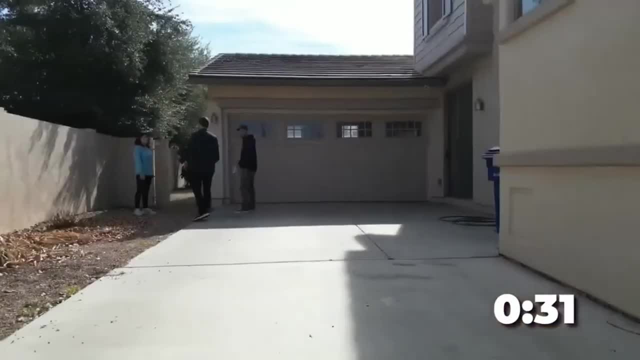 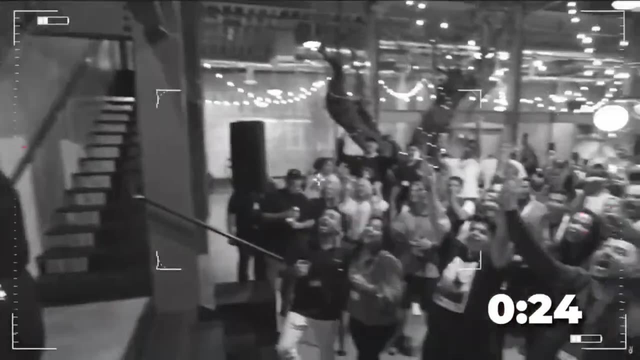 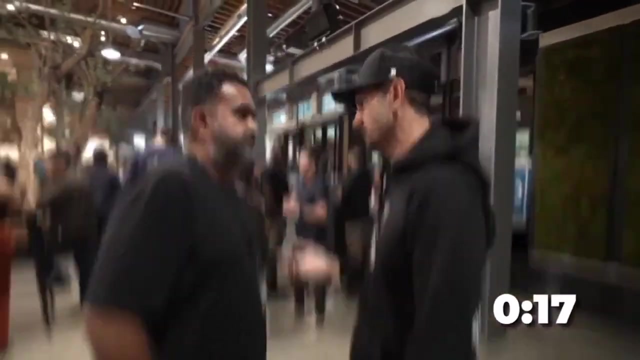 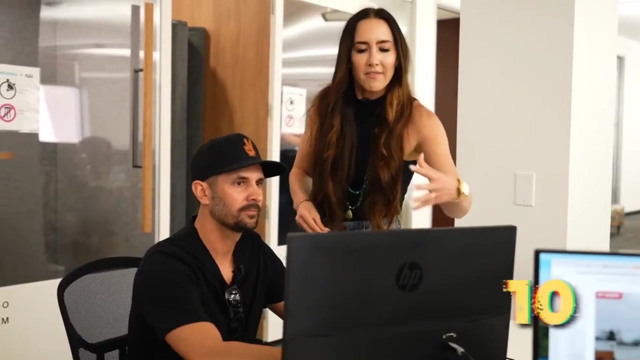 Pace Morby is the guy for all things real estate and he does it all with something called creative financing. It's going to be everything and anything you could ever want to know about creative financing. When I watch Pace, you know what I see. I see a guy who got a whole universe of humans who told 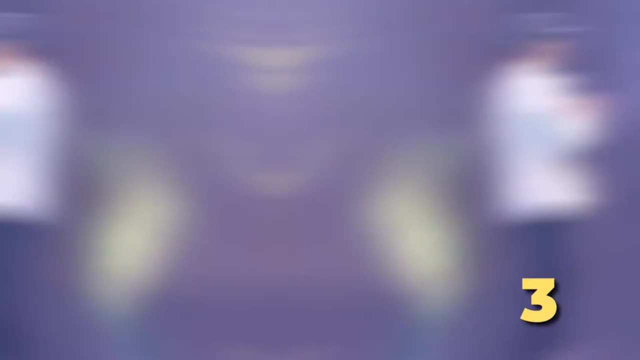 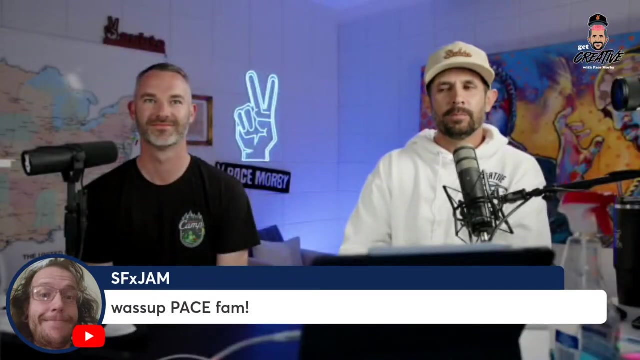 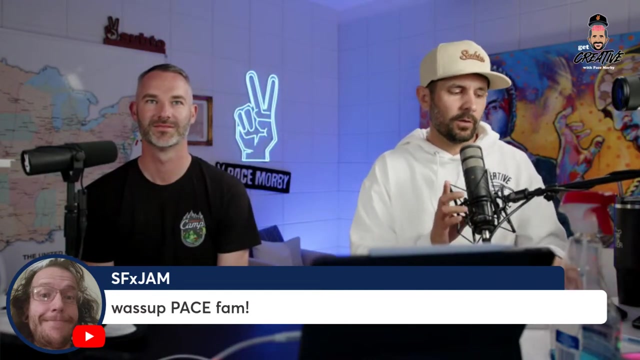 him you can't do it that way. And he said: f**k it, Watch me Yo. everybody, Welcome to Get Creative Podcast. I'm here, joined with Jordan Wittenberg, to my right- probably your left- And we're going to be hanging out here for the next 40 minutes talking about 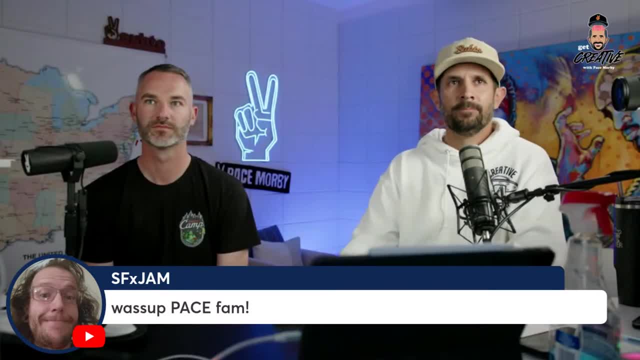 creative finance. Any questions you guys have in the comments today, Um, my team put a thing in the side, or the title of this called how to calculate terms, And I'm not going to do that today, And the reason being is I've got a. 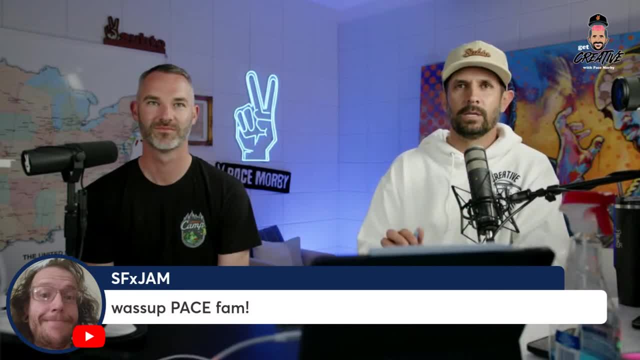 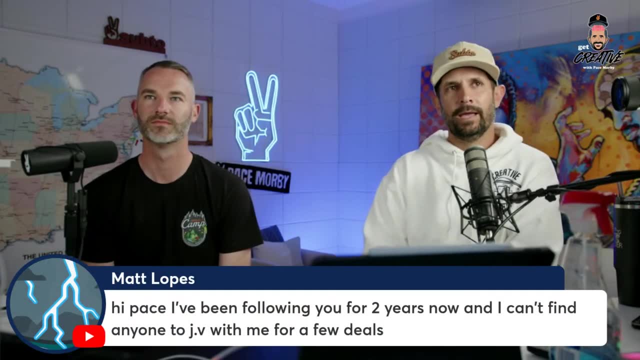 so we'll switch it up. I'll do how to how to calculate terms next week, But today we'll do a little bit of Q and a. ask me whatever questions you guys have, We'll jump into it. I'm checking this out. Matt Lopez says: hi, Pace, I've been following you for two years now. 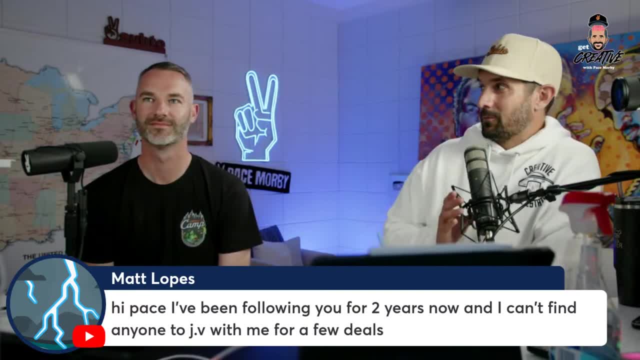 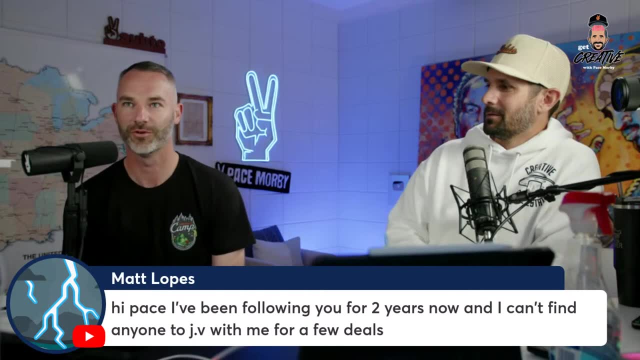 and I can't find any one- to J J B with me for a few deals. Is that even humanly possible, Jordan? It's not. If you go in your free Facebook group and scroll for more than four seconds, Like seriously, Yeah, I mean, they're everywhere and they're sub two. 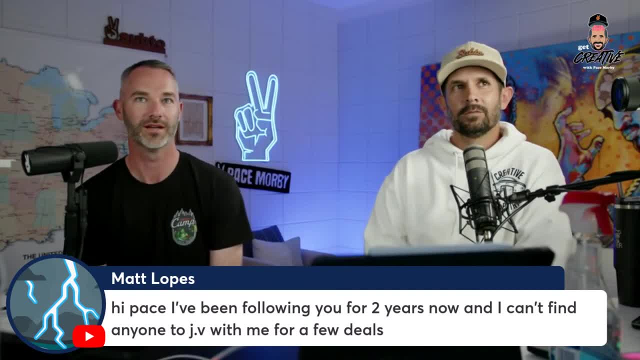 And they're everywhere that will partner with you and guide you along the way. So, Jordan, I almost feel like you should rephrase that statement by saying: Pace, I have been following you for two years and I've done everything out of my in my power to avoid J V with your students, And I've been very successful. Um, I can tell. 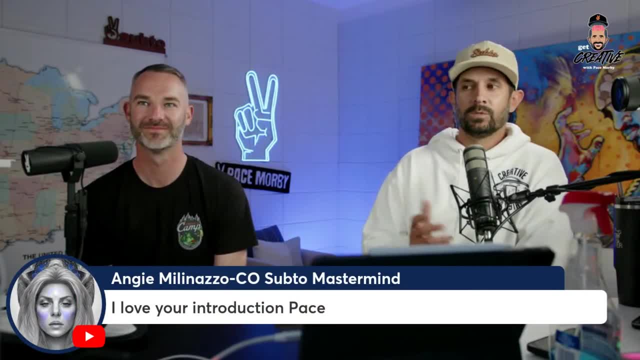 you right now, Angie Milanozzo in the side chat right here. Um, somebody I've J J B deal. uh, done J B deals with multiple times. She's a great leader in sub two. She has done probably a hundred plus deals with people. 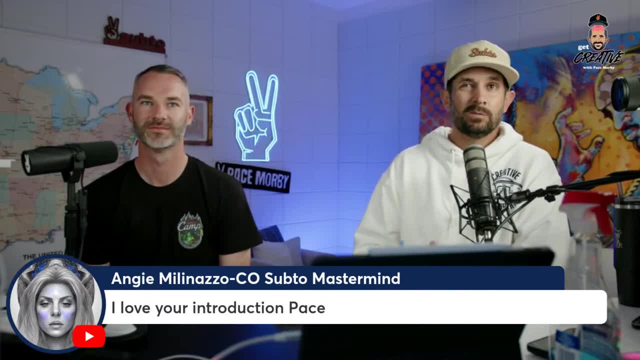 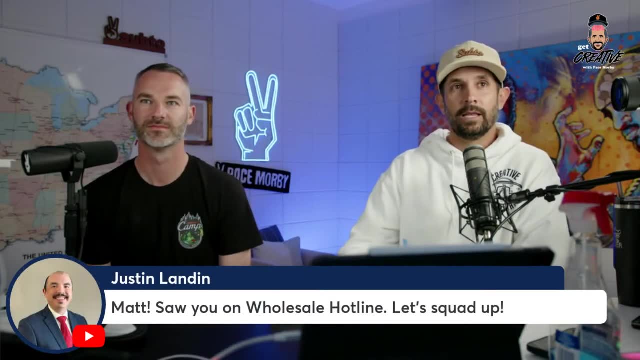 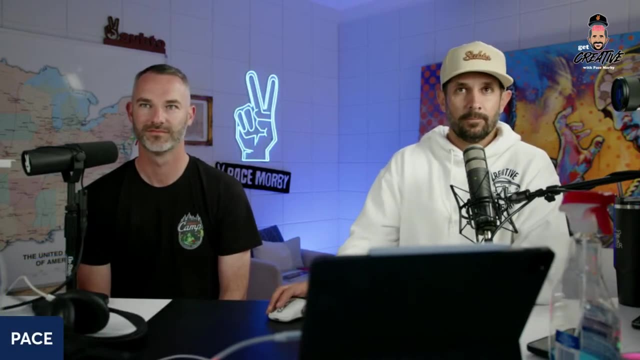 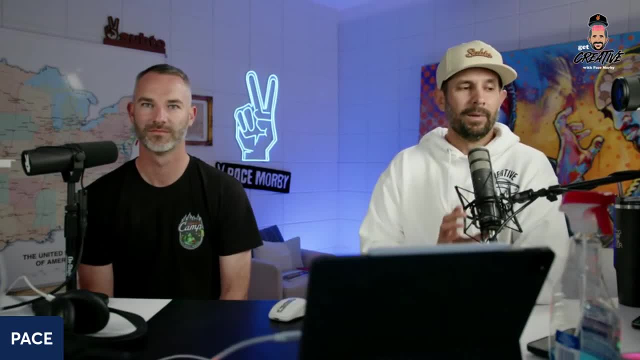 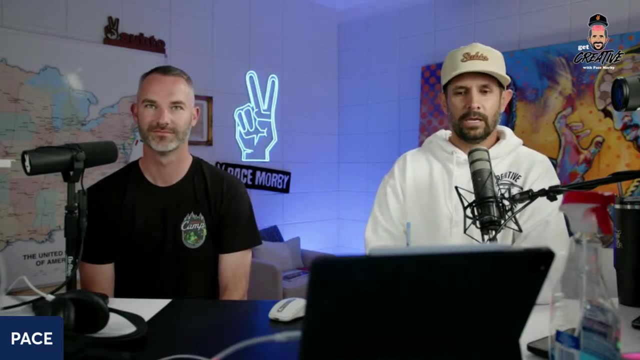 right here in get creative guys. Thank you so much for coming in on Monday nights. By the way, our podcast is now top 50 in the nation. Get creative is top 50 in the nation Podcasts um regarding most downloads, So thank you so much for doing that. 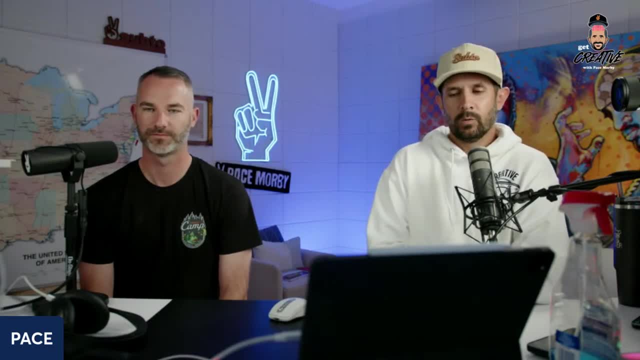 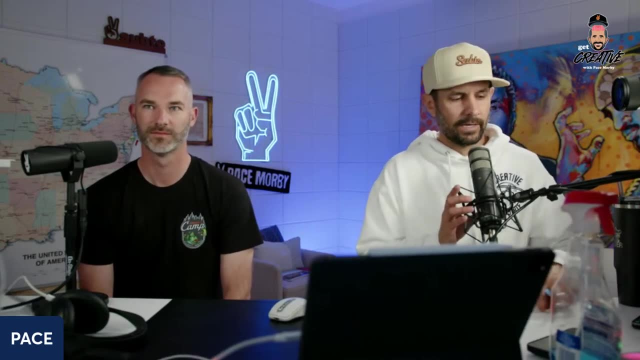 Showing up, downloading the podcast, helping out, uh, spread the word, all of the things. we just closed on a deal today. Um, that deal was a J B deal. Actually, it was a deal that was brought to me by Jordan. Ray is in the sub two community, He's in Montana and he knew that. 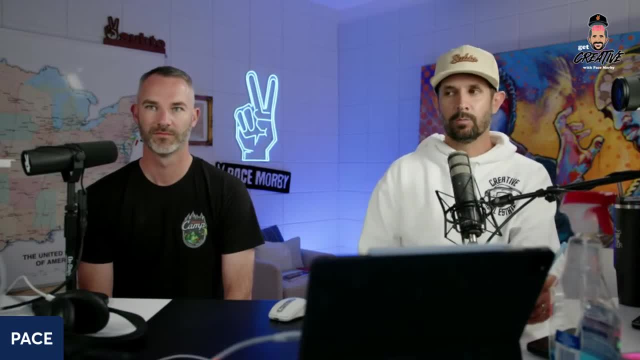 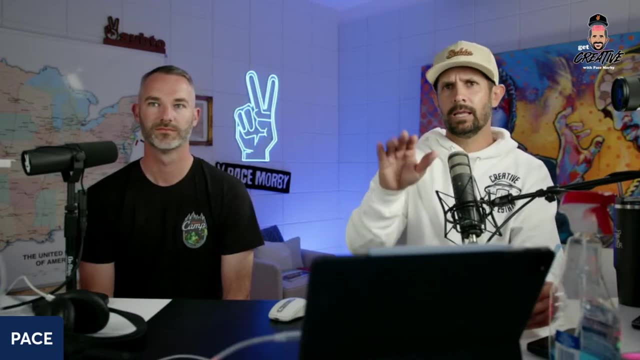 I was buying in Kalispell, Montana last year. He brought me two RV parks. So let me give you guys a little bit of education. Whatever you guys need, please let me know in the side chat. We'll do a little bit of Q and a tonight, whatever questions you have, wherever. 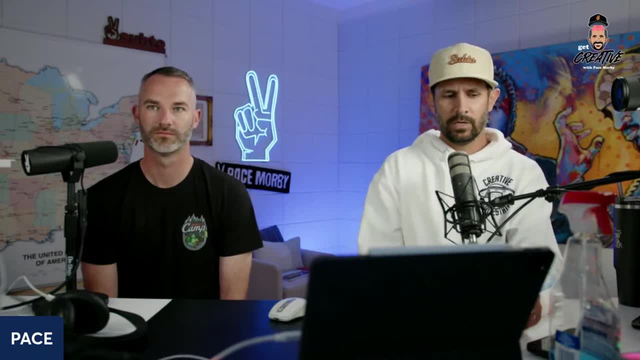 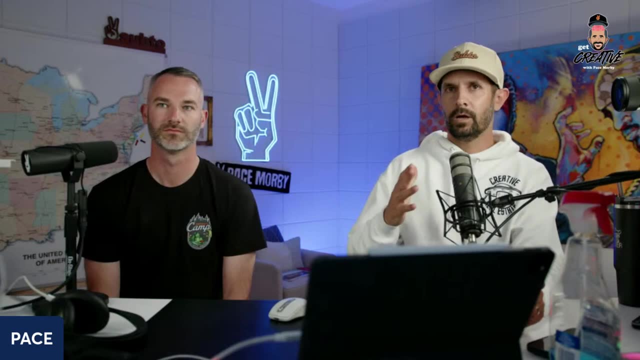 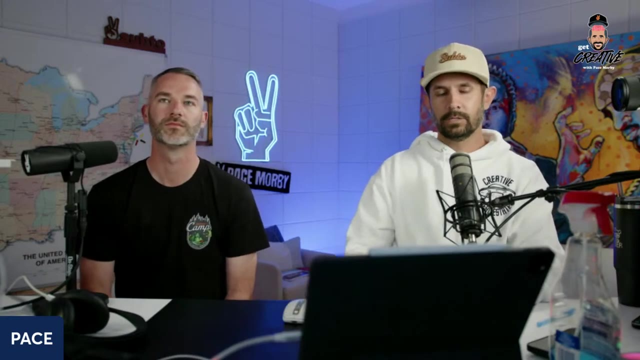 you're stuck, say it in the comments. We'll give you a little bit of advice. We'll be on here for 40 minutes. So Jordan Ray's brings me these two deals and the structure of this deal. Um, it's two RV parks. I'll show them to you. They're actually really good, great locations, And let's 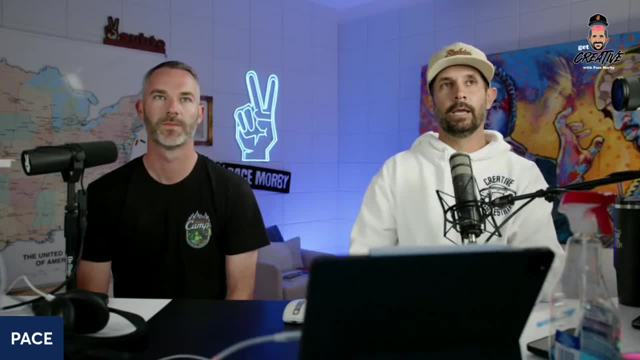 see, Glacier peaks is the one that I now own, And um Glacier peaks RV park and campground dope. What's somebody using Google AdSense to beat me out? This is not cool. Check this out, guys. This is not cool. We're going to have to beat these. 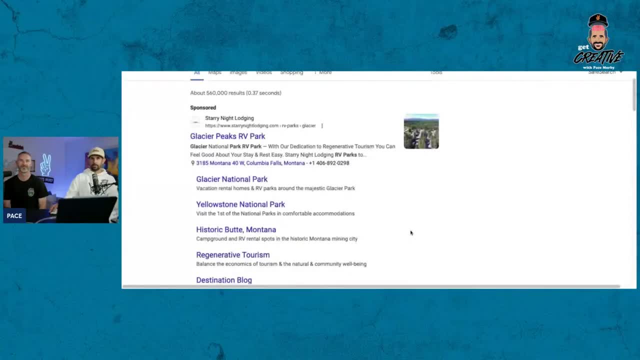 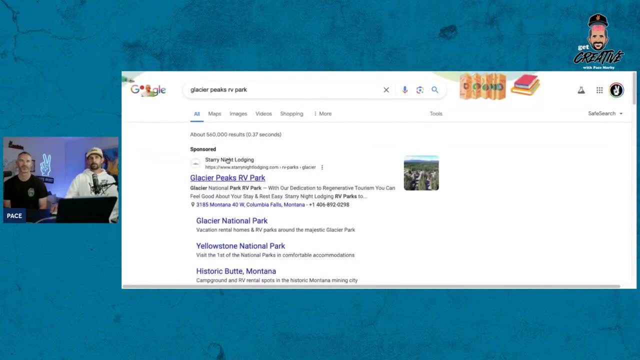 people out. You want me to show you how I'm going to beat everybody in Kalispell on these RV parks? Check this out. I Google Glacier peaks RV park and starry night lodging beats me out because they sponsored it. That's not cool. I don't like that. We're going to see what we can do to beat. 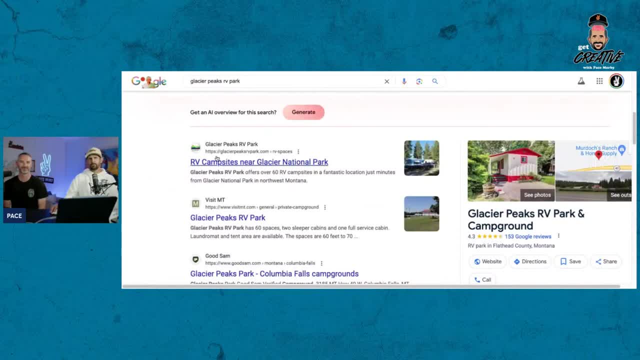 them out. Um then, look, RV Glacier peaks RV park. That's me, Dope, Let's go over there. This is our park. I'll show you guys the location. I could not have gotten a better location, Unbelievable location. 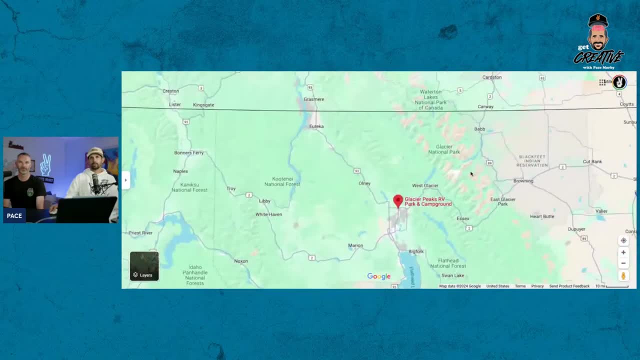 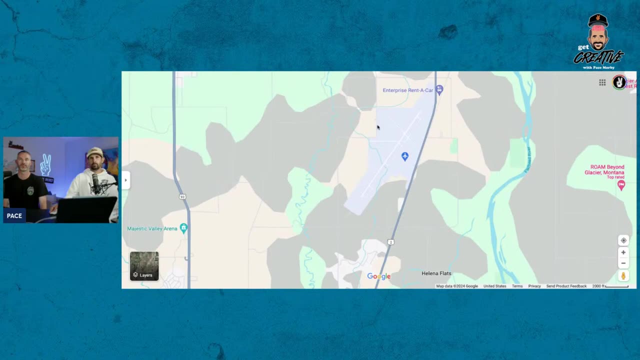 If you look at the whole Valley, Glacier national park is up here to the right. The airport is right here in LaSalle Boom And you leave the airport to go to Glacier national park. You have to go up the main road and go to the airport And you leave the airport to go to the. 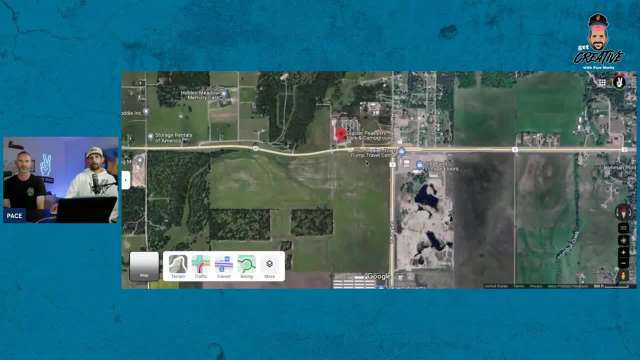 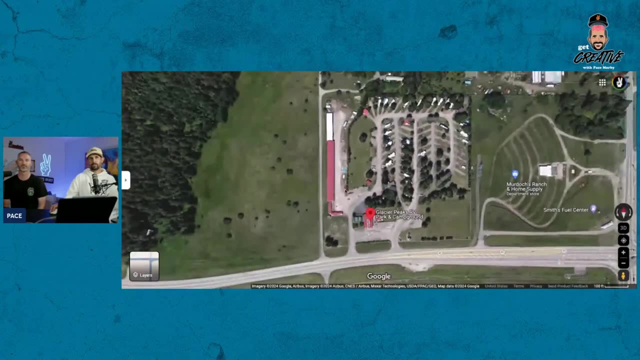 airport And you leave the airport to get fueled up at the last gas station on the way up to Glacier national park. And guess what? That gas station is across the street from my RV park. We've got 40 storage units on that RV park and about 85 pads here. We bought this for $5 million on seller. 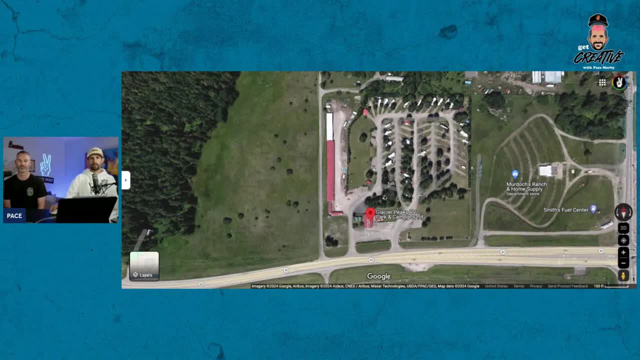 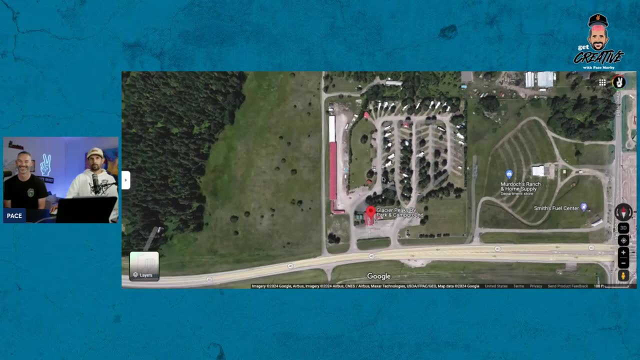 finance. I did not get my credit check. I did not use a bank. I did not use any of my own money. Your W2, though I do not have a W2.. I don't know that I would be a good W2 employee, to be honest. 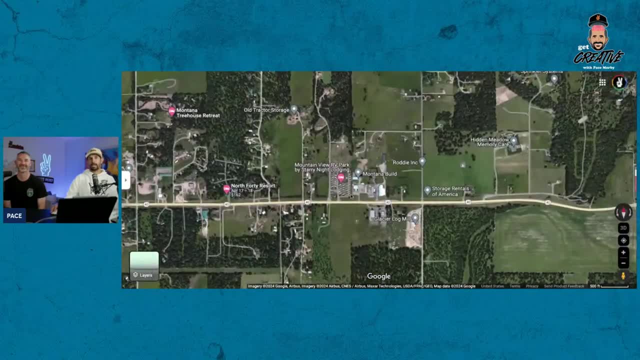 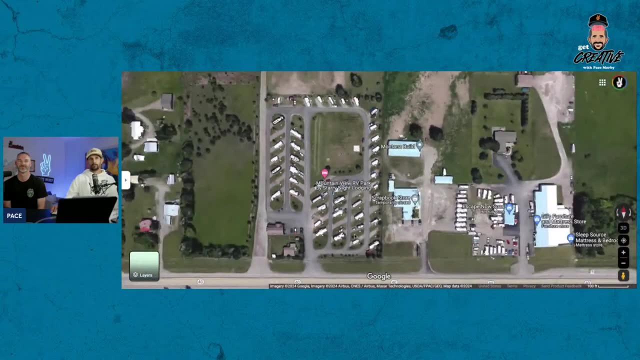 with you, but that's um good good to bring that up. And today we closed on this little cutie right here, Mountain view RV park. Um right, Same owner that sold it to us Name it is Eric. This now has a mini. 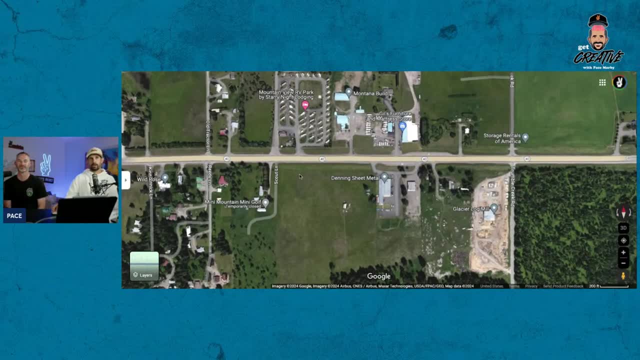 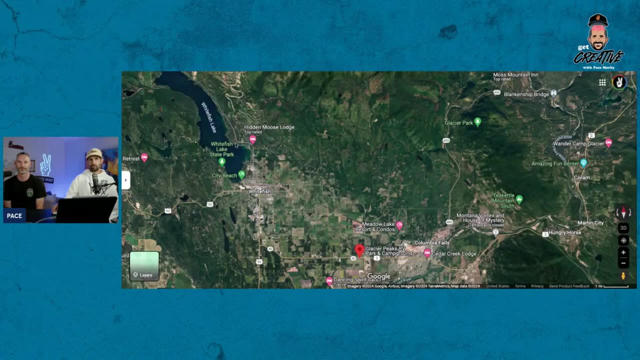 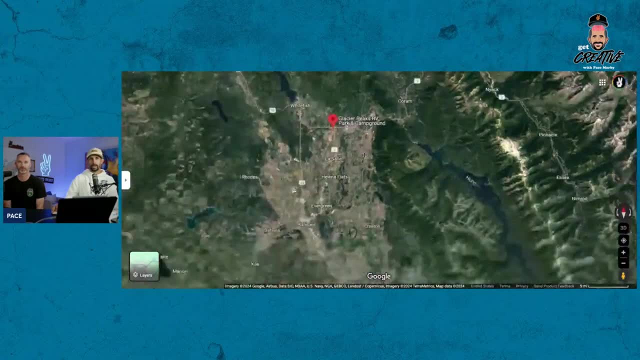 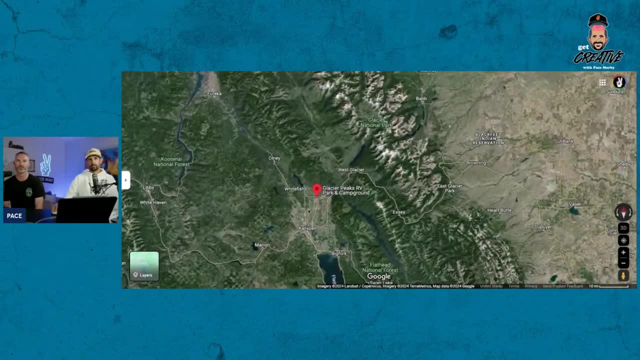 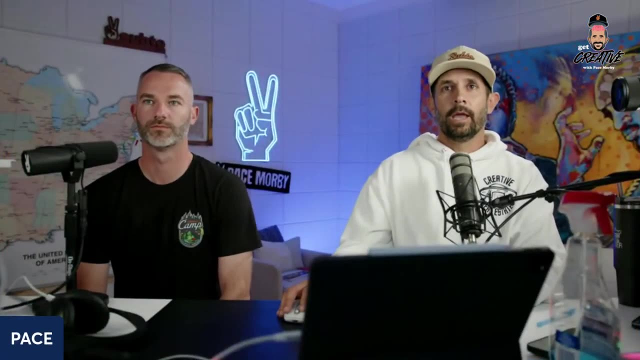 white fish and Glacier national park, or unbelievable, unbelievable. So I got both of these bad boys. It was brought to me by um Jordan Reyes, who lives down in Missoula, And um, here's what happened. Eric the seller is in a bad financial situation in a different business. 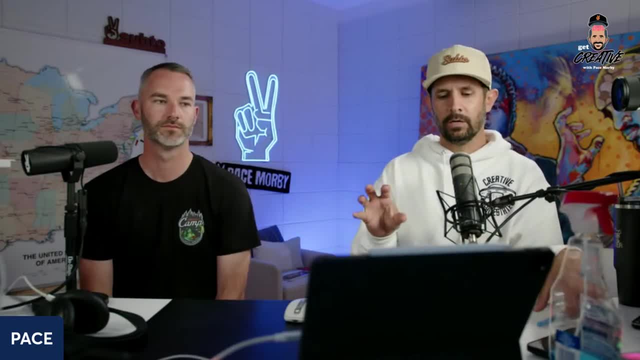 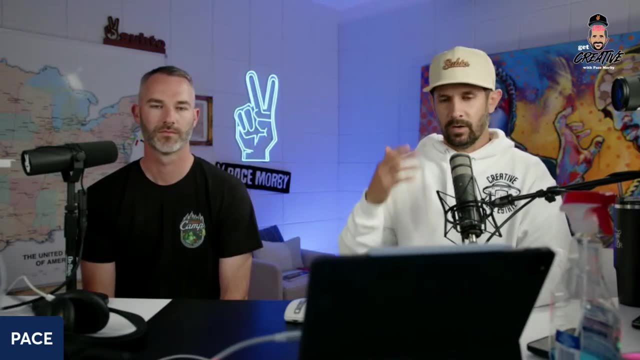 So Eric owns both. those are RV parks. a year ago He decides I'm going to go to a different business. I'm going to list them. His broker can't sell them. We reach out to the broker multiple times. We offer seller finance. No, no, no, no, no. Then the listing falls apart. Jordan Reyes reaches out. 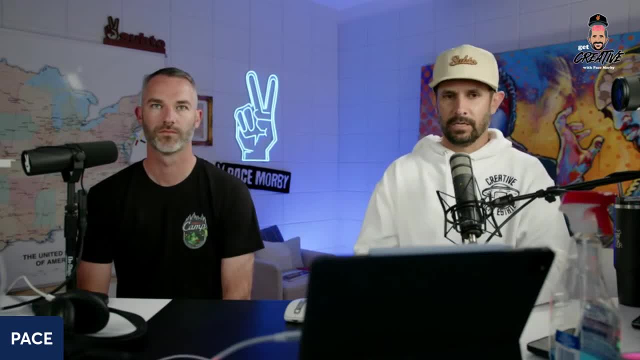 to the seller, Eric, and says, Hey, I'll buy these on seller finance, We'll save you a bunch of money on taxes. We'll pay you your number. And there goes the negotiations. The negotiations um lasted about three months going back and forth with all sorts of structures. Let's do a contract. 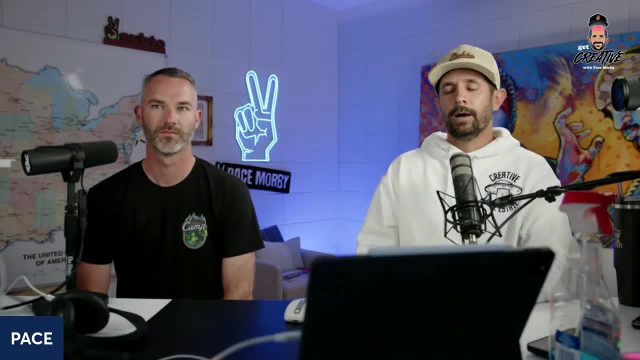 for deed. Let's do a no money down, Let's do a this, that and the other, Um, and ultimately the first park, the one I showed you first, is a $5 million purchase, 5% down, So $250,000 down. 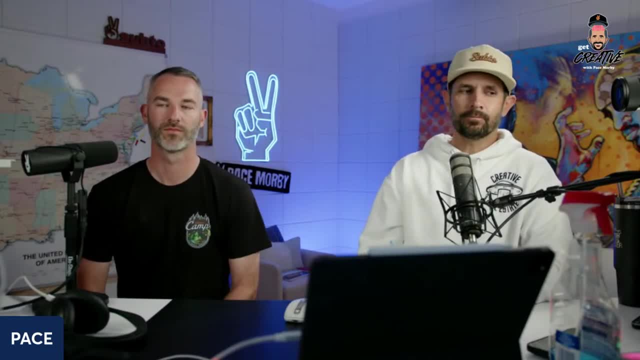 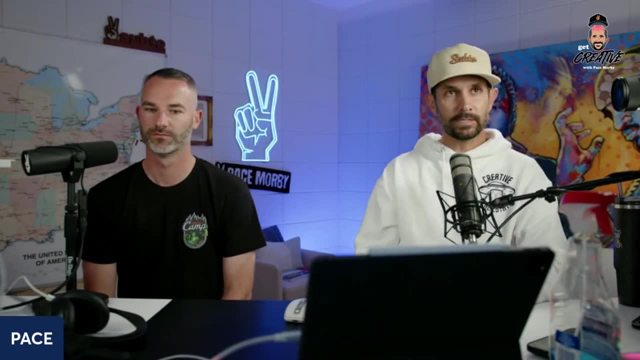 I did not use my money for that. I brought in a private money lender and that park is already booked out for like a year and a half. It is booked out, solid things, cash flowing, I think, our net cash flow on that thing in the peak summer months. we're netting something like 30 grand a month And then in the winter months we basically break even. So our average month is about 11, to $15,000 a month. Net, net, net in my pocket, net, net, net, And then the other park. 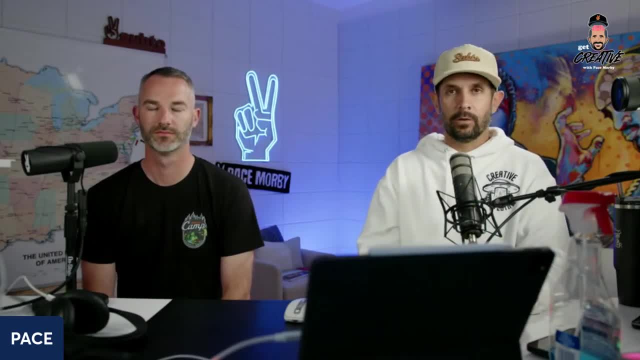 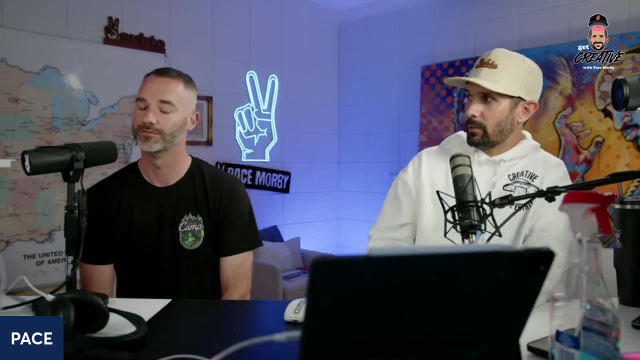 the smaller one we closed on today. You guys can look on my Instagram story. We closed on that today. Um, that one we are actually doing the BRRRR strategy on. So as much as I talk crap about the BRRRR strategy, I sadly am doing the BRRRR strategy right now. Um, okay, This is great. 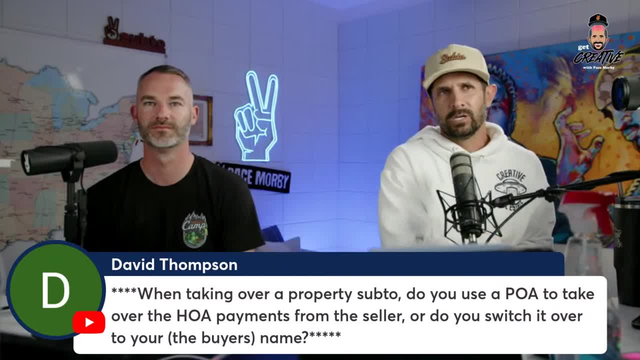 David Thompson says: pace when taking over a property. subject to: do you use a power of attorney to take over the HOA payments from the seller Or do you switch it over to your buyer's name? Yes, You switch it over to this, So there's an. 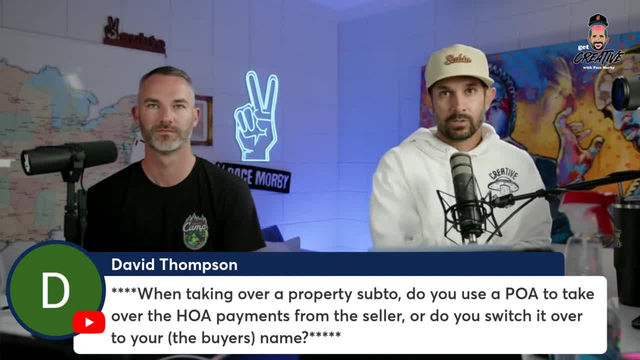 HOA transfer document. A lot of times it's at escrow. The escrow officers actually do this for you. So, yes, that is correct. You fill out cause you're the new owner. by the way, David, you are the new owner. I think that's probably one of the hardest things for a lot of people. 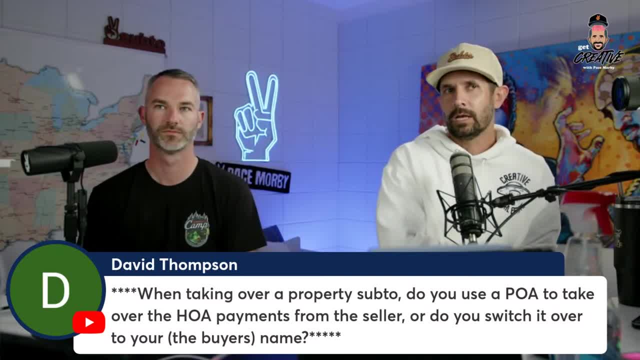 to understand. They're like: wait, you bought the property subject too- but the owner still owns the house. No, they do not own the house, My friend. you own the house. You, oh my gosh. So many times in my life that when I go to re-explain it, I go: wait, I've explained this. 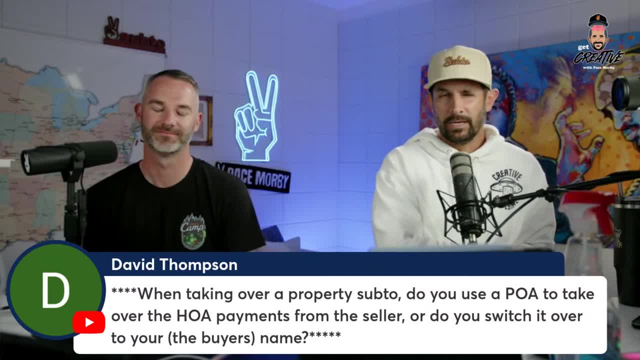 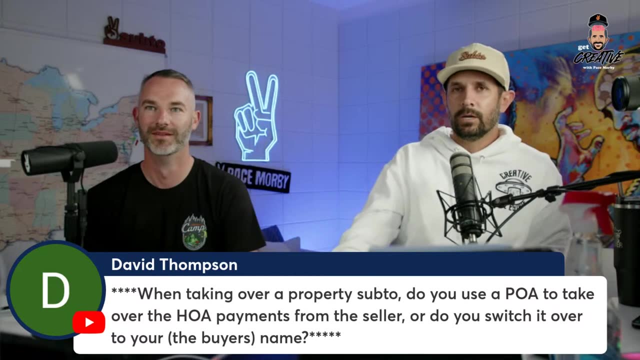 That means I probably have. I've not explained it properly. I did not know. I didn't do it right Other than otherwise, David Thompson would know the answer. The reality is I have to be a broken record, Like Don Walker says, 10,000 times, So everybody can understand. 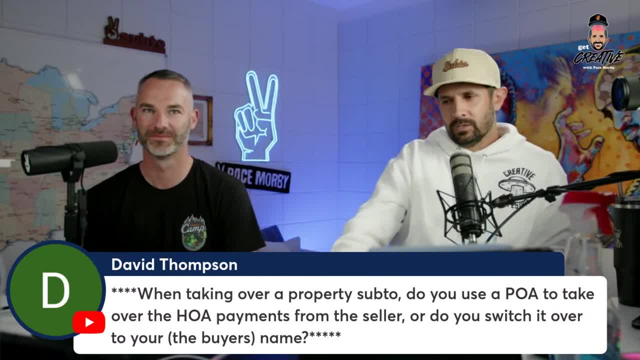 the owner of the property is you, David Thompson. So when the HOA is wanting to know who the owner is, you simply just tell them: you're the new owner. It's really not that hard right? You, it's really it's. it's actually so simple. 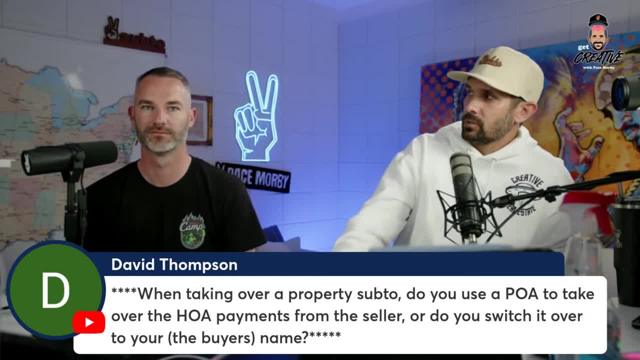 that people overcomplicate it Cause they're like: there's no way. it's that easy. That's all it is. By the way, you guys, uh, Jordan Wittenberg, reach out to him. What's your Instagram at, Jordan Wittenberg? Okay, How do I spell that? 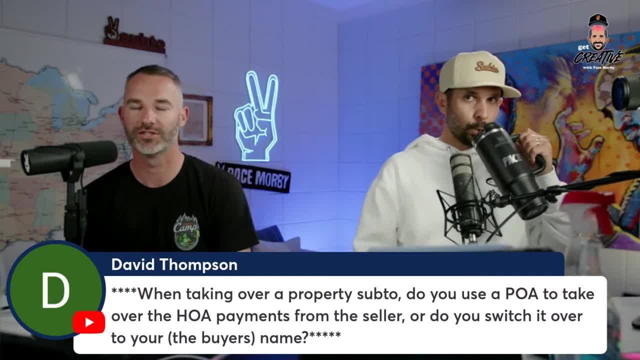 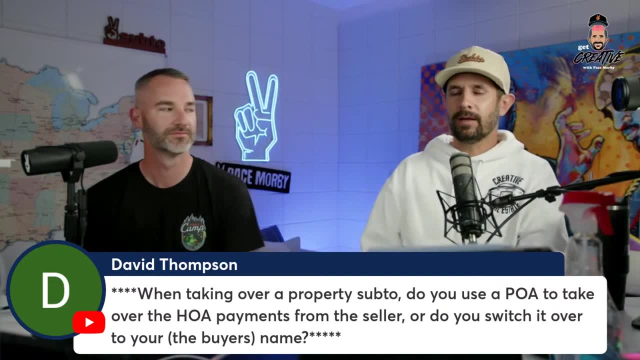 Jordan. J O R D A N Wittenberg. W H I T T E N B U R G. Jordan Wittenberg last year got a $95,000 assignment fee on a door knock Man, that was a ride. Yeah, We talked about it today. 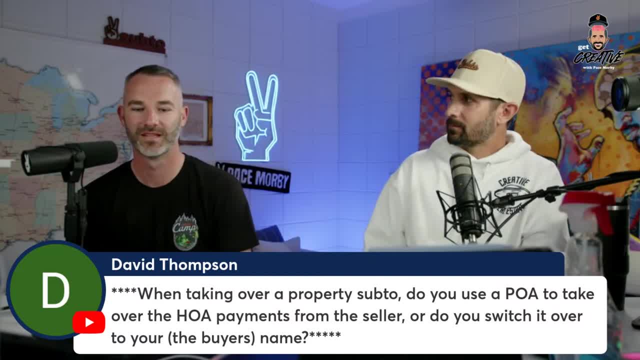 $95,000 knocking a door? Yeah, Getting out of your comfort zone can pay off. You're persistent with it. What was the biggest lesson you learned on that deal with with, uh, William, Like I said, where, where there's a will, there's a way. 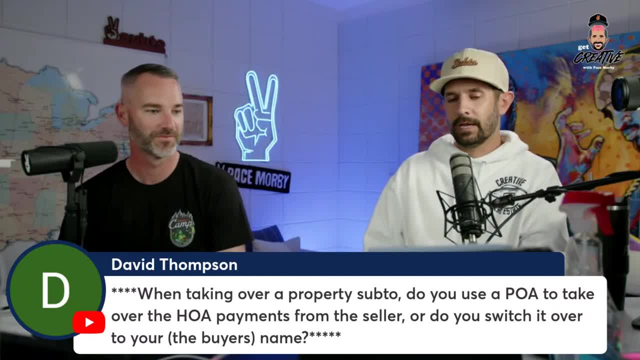 Where there's a will, there's a way. Now, this deal that you did last year, the $95,000 assignment fee that you got. you sold that deal to Mike key in Idaho, who also was in sub two. He's in the middle of flipping the property right now. When you got that deal, 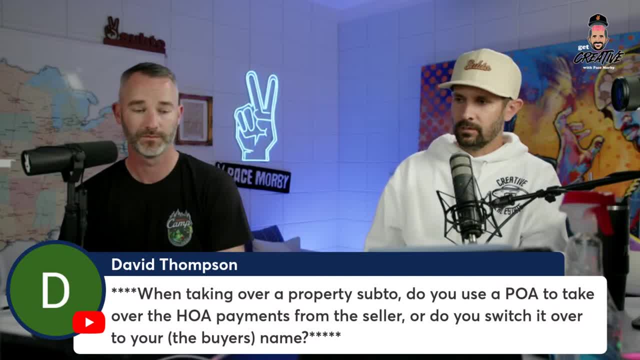 it was like two days away from getting foreclosed on. You jumped through 85 hoops to to stop the foreclosure and then 8,500 hoops to get get the thing actually sold to Mike key. I feel like one deal gave you like a masterclass on foreclosure, man. Yeah, It was a crash course. 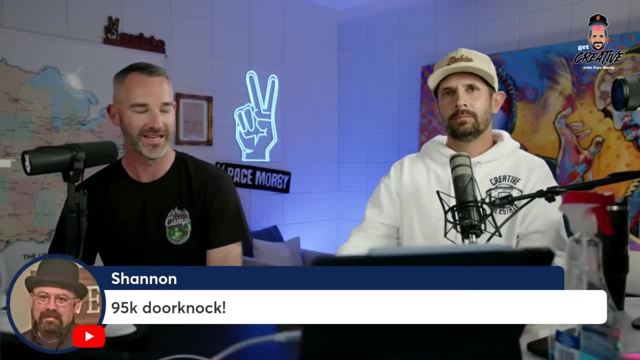 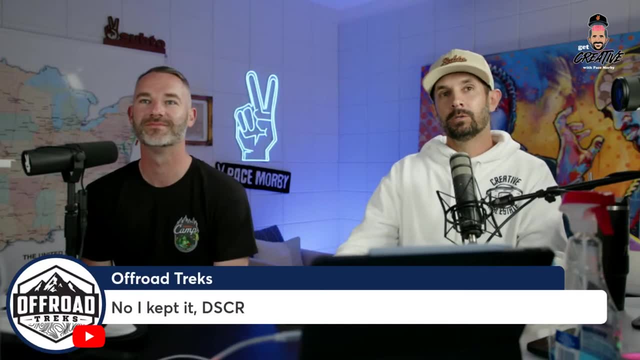 Yeah, Anything that could have popped up did, and just navigated our way through it throughout the whole process and found a way to get it done. Oh, check it out. Yeah, Is that my key off-road treks? He says no, I kept it. DSCR. 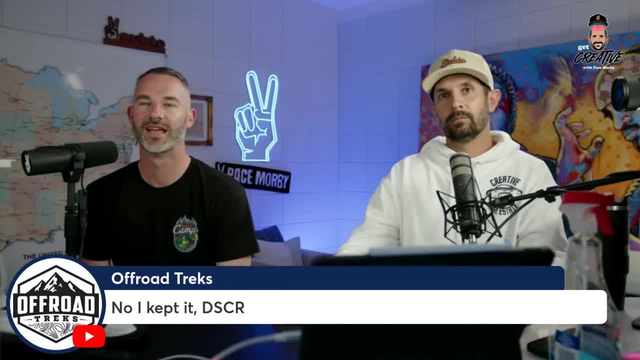 Oh, he's going to keep it. I don't know. I don't know if that's my key or not. He had talked about maybe keeping it Um, and he was between, but he's fixing it up. I know that. 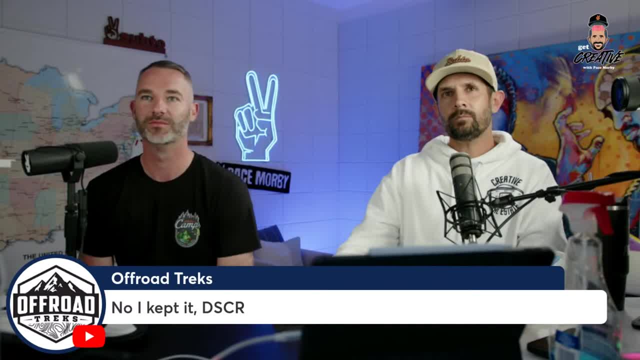 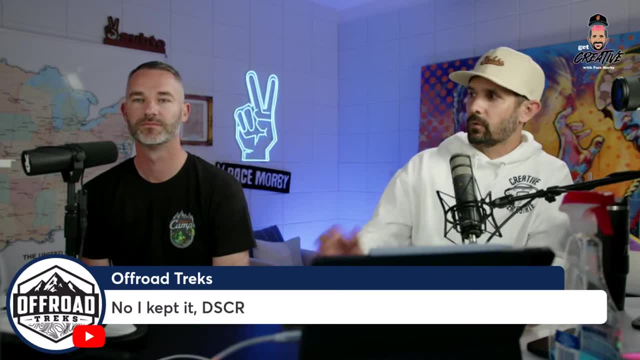 Okay, cool, But he was between buy and hold, or or it was: um, it's a great story, An awesome story. You made 95 G's on the deal. You helped the seller that nobody else could sell. In fact, what was the first? you knocked the seller's door. 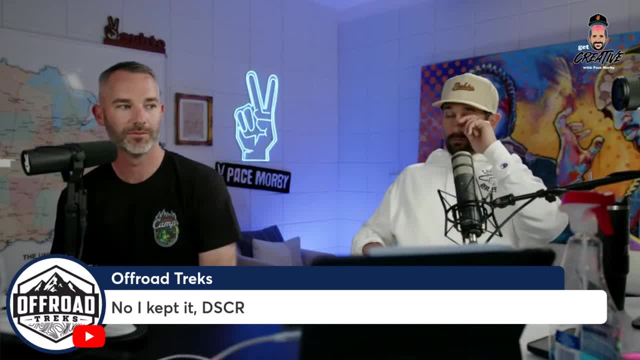 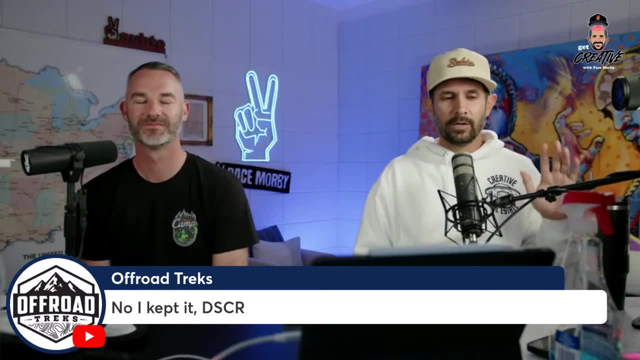 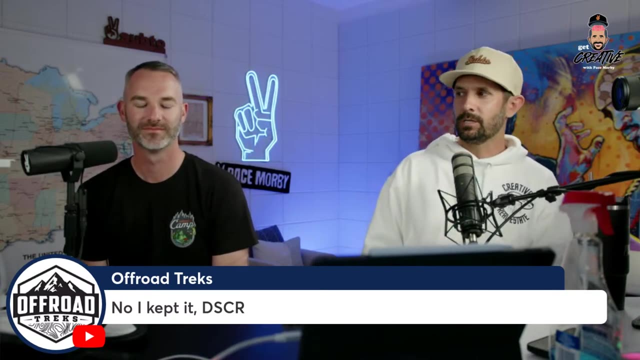 Yeah, What was the first words he said to you? Don't waste your time, It's hopeless. Didn't even say what's your name, Didn't even say can I help you. He opens the door and tells Jordan: don't waste your time, It's hopeless. And then you proceed to go and help the man and make 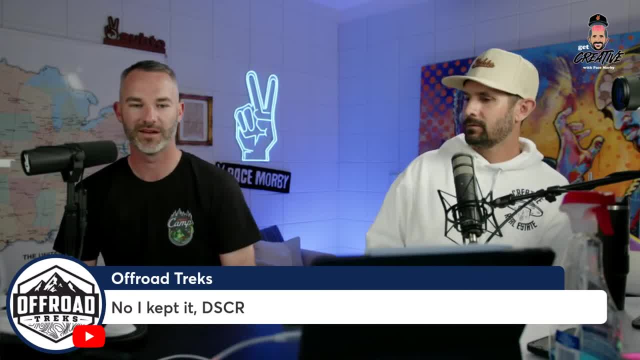 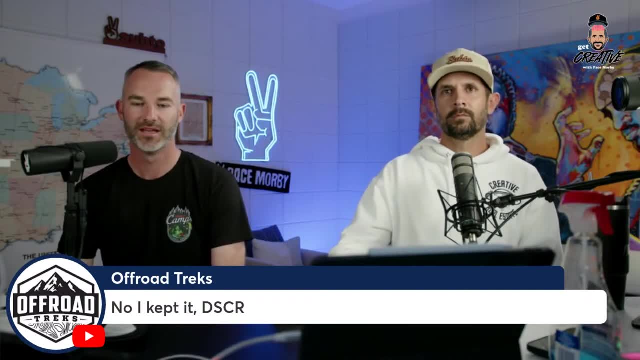 95 grand. Yeah, I just said I'm here to solve problems. He invited me in and explained his whole situation in his living room. It was about an hour talk And uh, he knew I was just there to listen to. 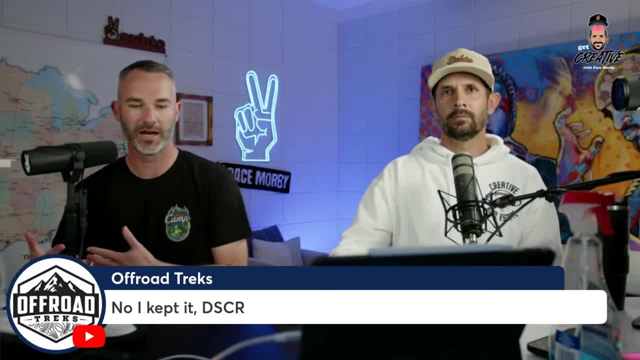 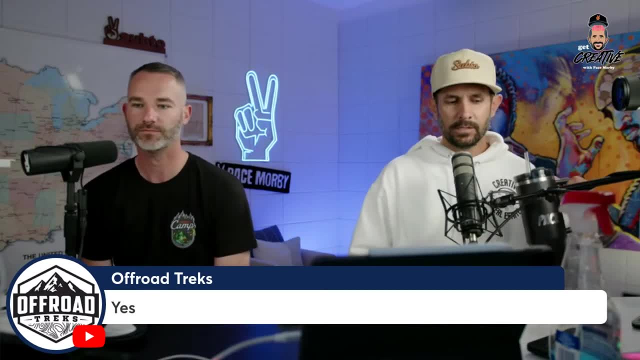 him and see if we could figure something out. I didn't know if I could yet, but I wanted to at least listen and see if there was something he could do that he just wasn't aware of yet. You know, what I love about this is that we you met. how did you meet Mike key? Was it a meetup? 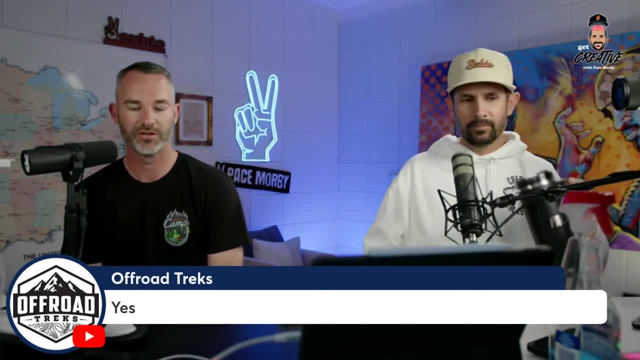 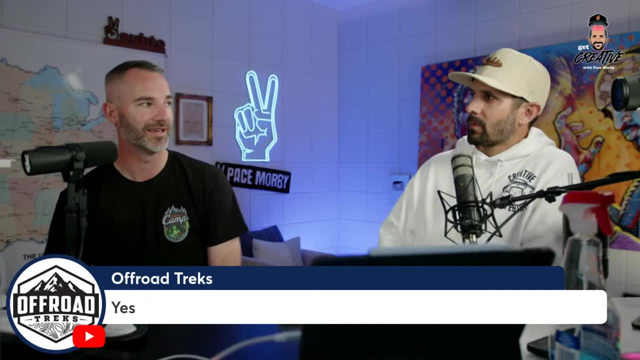 I met him at a sub two meetup in Boise- Yeah, Shortly after I joined last year. And um, and then I at that limitless event, uh, we talked about that deal more in depth And uh, this one just happened to match his buy box like perfectly, And uh, 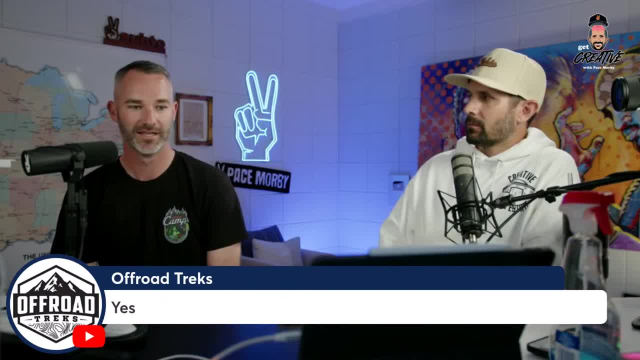 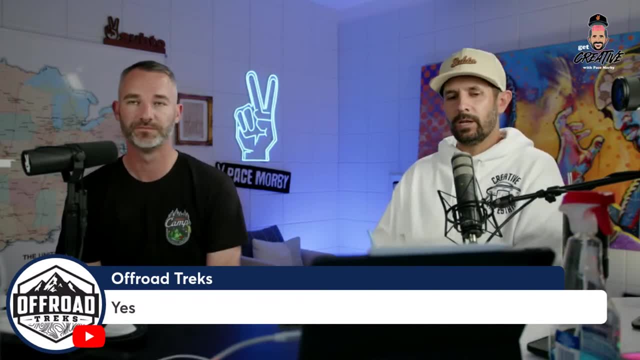 so it was just a good fit And I I pitched him the deal and it was what he was looking for And it was a good. it was a win-win for everybody. You know, what's cool about that is that people are like: why do you go to people go? Why do you? 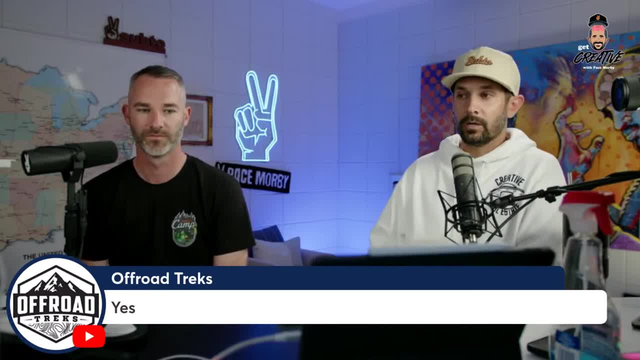 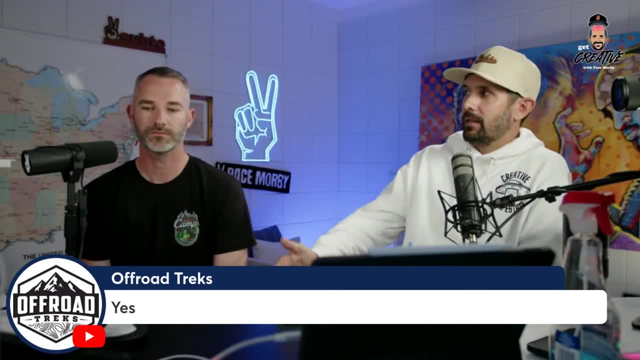 always do and go into meetups. I my friends like, why are you always going to meet up with my bro? The deals get done At meetups, They freaking get done at meetups. I mean, if you, if you had not seen my key, that 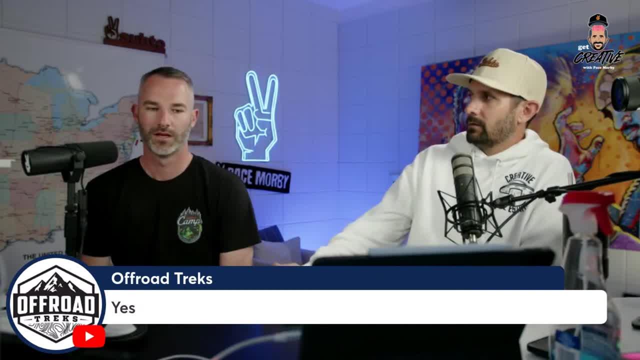 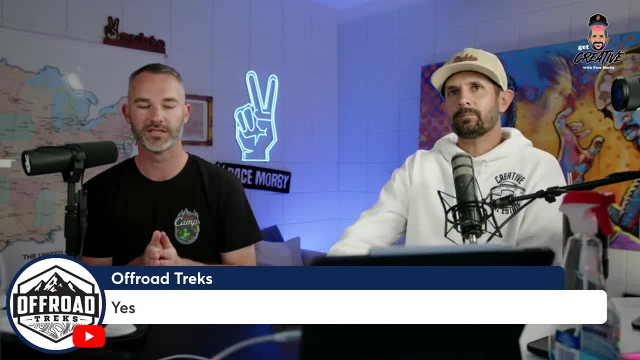 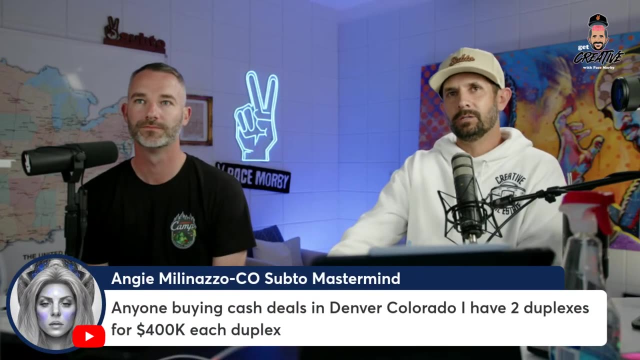 day at limitless. would you have sold that deal to my key? I would have reached out to him. Um, just so, maybe. yes, Yeah, But it helped talking about it in person. Um, there's a, there's value in that physical proximity. Yeah, I love that. Um anyone buying cash deals in Denver, Colorado? 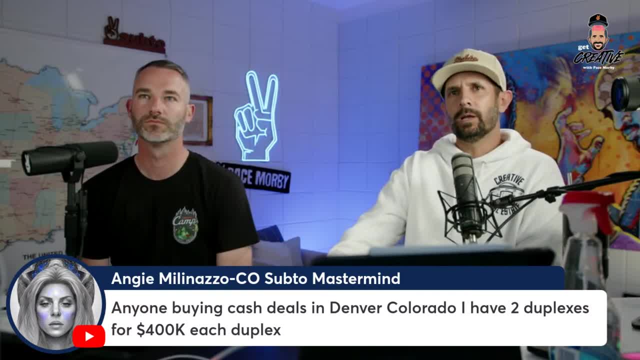 have two, two plexes- Whoa Two duplexes- for $400,000 each. So you're telling me, for a hundred grand a door I can buy a property in Denver, Colorado. That sounds like actually a good deal. Um, I imagine the rent rate on each one of those. 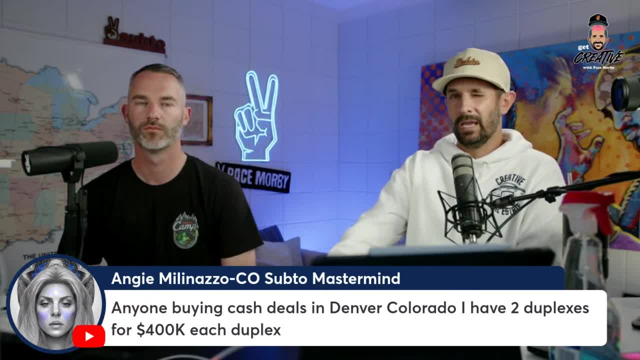 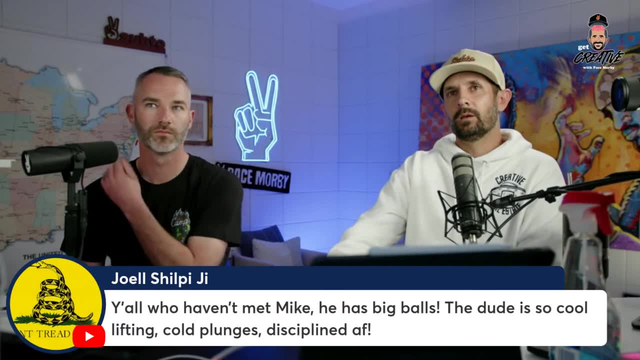 units, and if it's in Denver, those units could probably be 1800 bucks. Is that what you're trying to tell me? Angie Milanozzo? Um, cool, Yeah, this is great. Um, y'all who haven't met Mike, he has big balls. The dude, the. 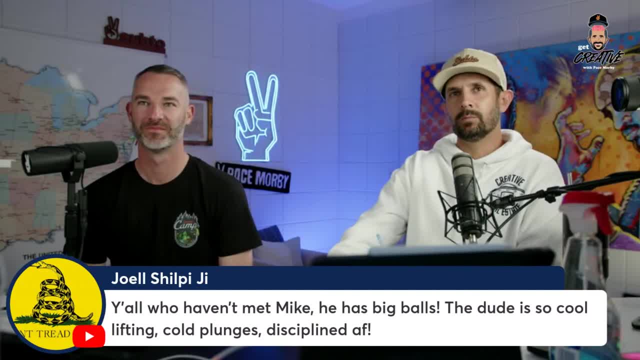 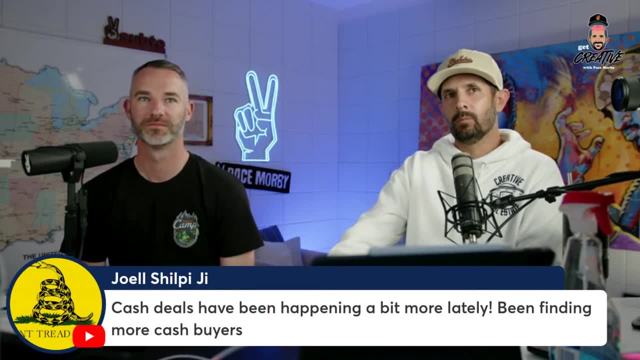 the dude is so cool, Lifting cold plunges, disciplined AF. I would say that that's true 100%. Um, cash deals have been happening a bit more lately, been finding more and more cash buyers. Cash buyers are back in the marketplace. They realize that rates are not going to be coming. 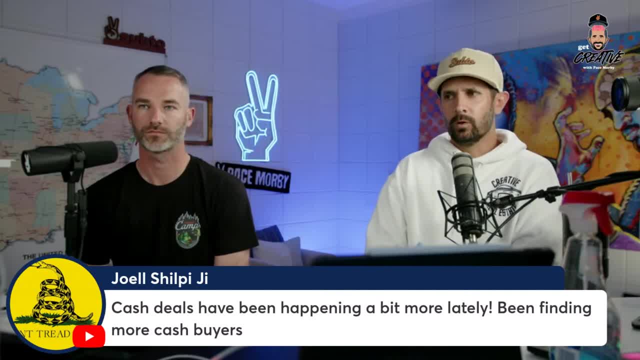 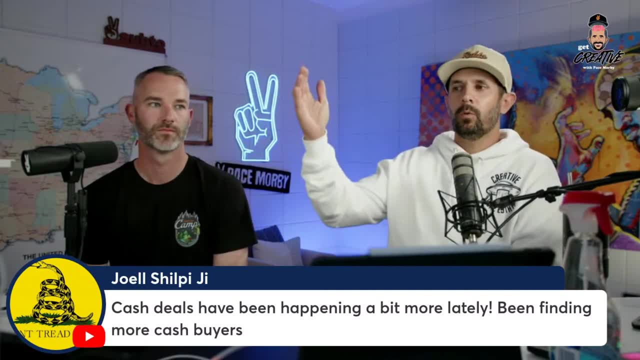 down immediately. but they realize rates will come down at some point, And so they're starting to buy more properties with the expectation that the market's going to go up when interest rates go down. And when is that? The best time to flip is when you feel like the market is going up or staying stagnant. 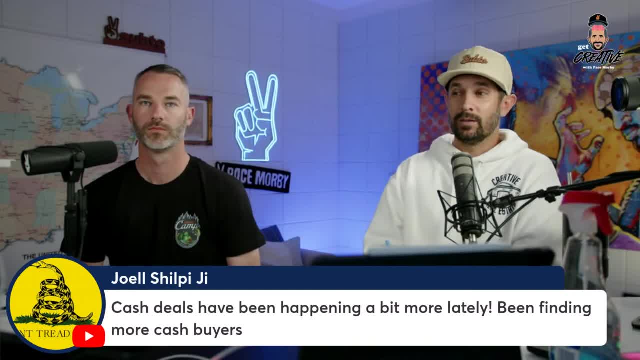 Um, definitely not in 2020, end of 2022, beginning of 2023.. A lot of people lost their butts in fixing and flipping because the interest rates were going up and the market was going down. Uh, so yeah, you're going to see a lot more cash buyers coming into the marketplace. 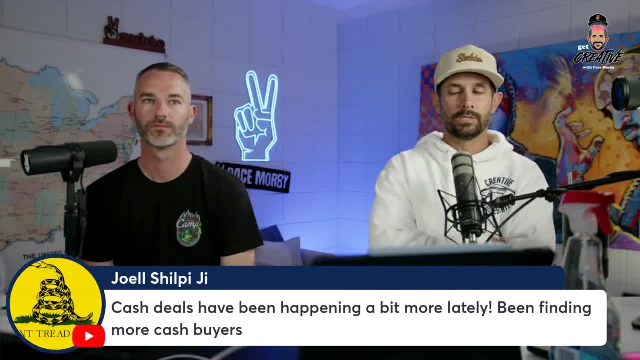 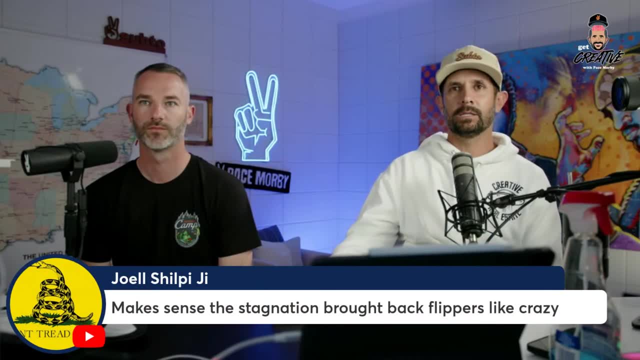 buying up a lot more deals over the next couple of months. So you'll see a lot. our community sub two will be doing tons more cash deals Over the next year for sure. Um yeah, max makes sense. The stagnation brought flippers back like 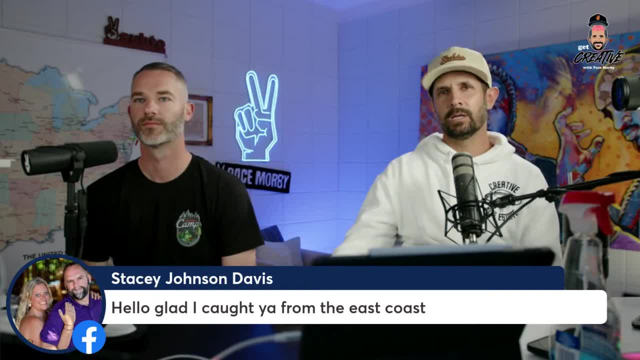 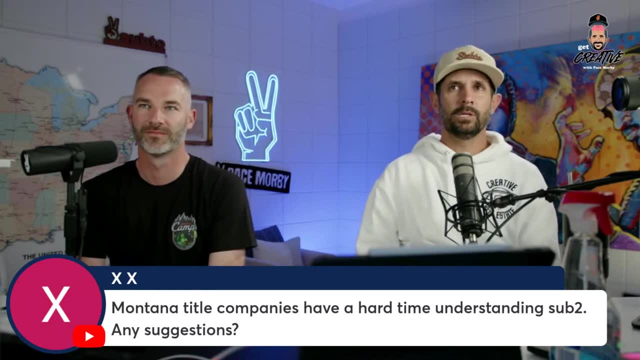 crazy. Um, all this is cool. Thank you, Stacy. She says hello, caught you from the East coast. It's 10, 15 at night. Um, Montana title companies have a hard time understanding sub two. any suggestions? Yes, Join the community and work with Montana students. that will get that put you in. 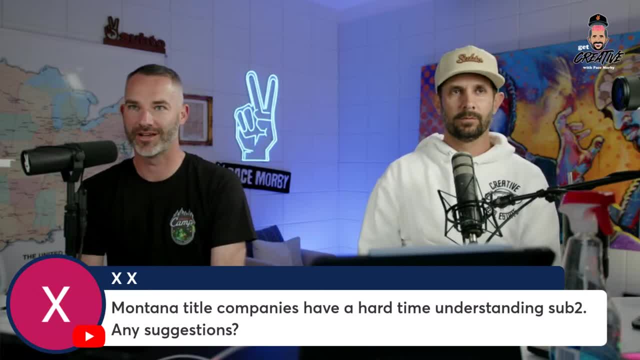 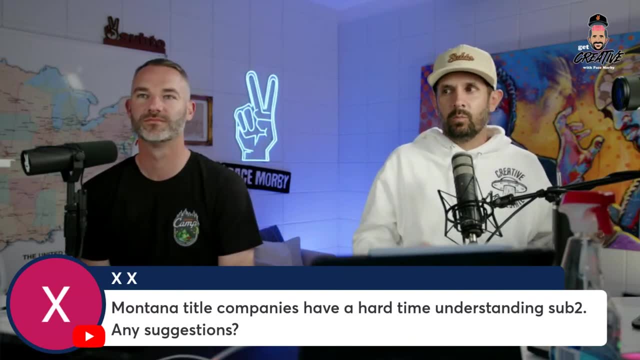 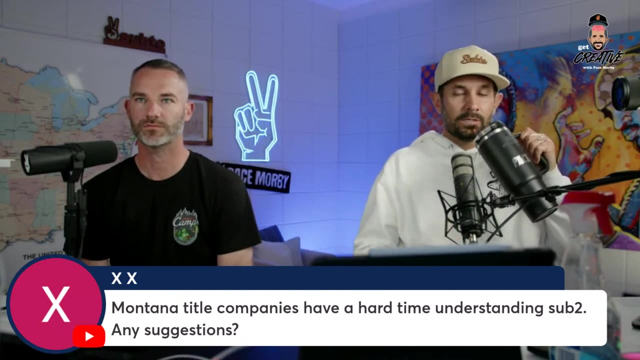 touch with the right title company, Jordan Reyes. shout out again: There you go, Jordan Reyes. I just did. I just closed with fidelity title in Montana a $1.4 million deal today. It's the same title company that did a seller finance deal with me and another same title company did a sub two. 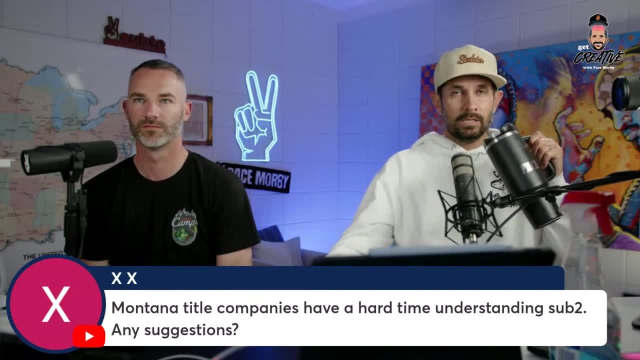 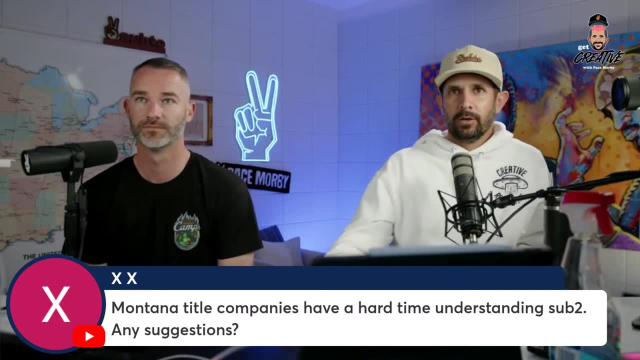 deal with me in Montana, the exact same city, the exact same title company. You just got to know the right people with the right connections and get good at explaining it and get a good explaining. There you go. That's a big part of it as well. Um, yeah, this is good, but deals have been. 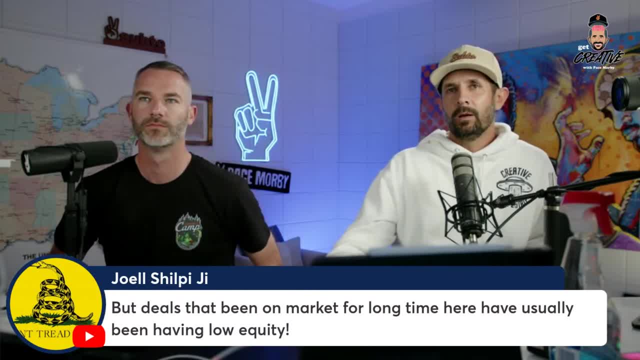 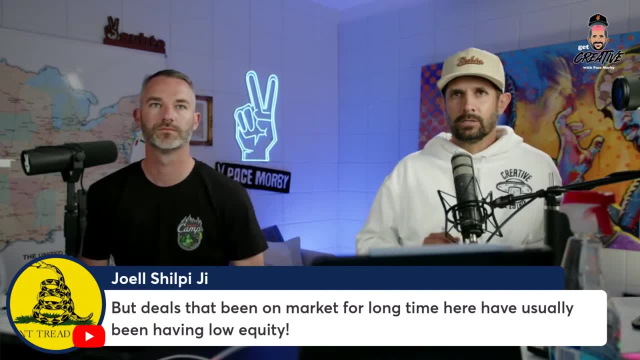 have been on the market a long time, have been usually having um low equity. Now what's interesting too is like the market has. the days on market is a really high. The average days on market is much higher than it normally is obviously the last year. 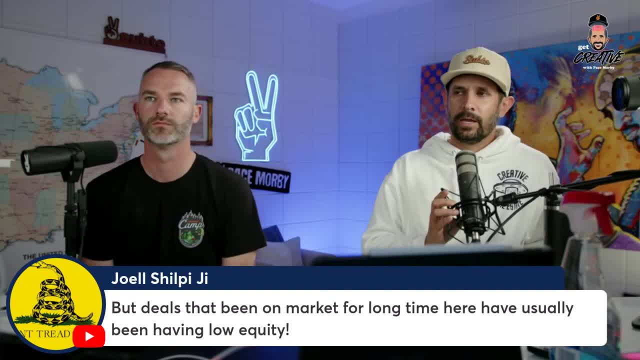 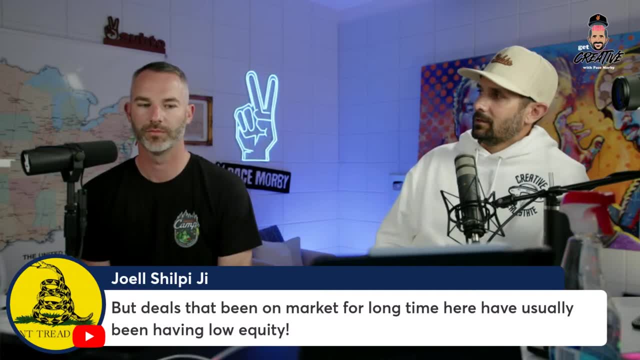 And so cash buyers are giving this um amazing success rate of low balling. In fact, we were talking to Donda today and she got a deal where she just goes: Hey listing agent, half the price, Let me offer half the price, Yeah. And they said yes. 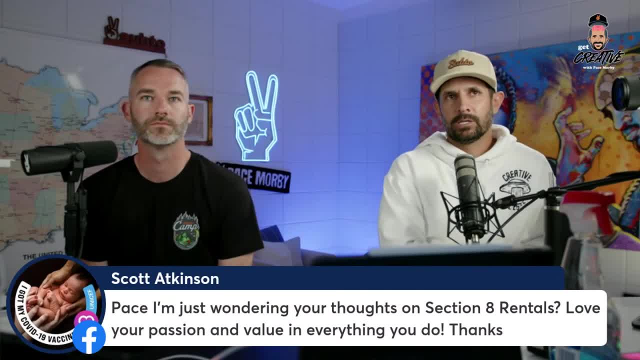 Hmm, This is an interesting thing. You guys are seeing a lot of ads for section eight rentals. Okay, guys, let's talk about section eight rentals. What is so exciting about section eight rentals? What? let you tell me. you know what it is. 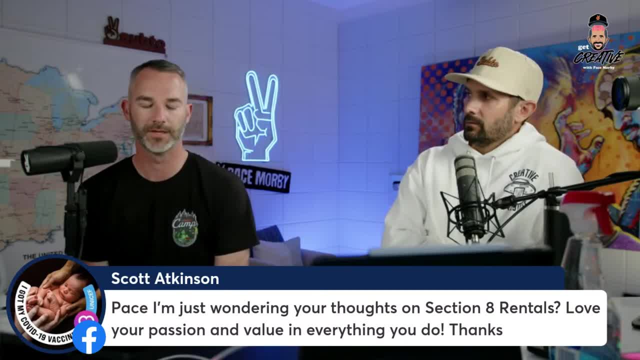 Oh, it's guaranteed government. It's guaranteed government money. People really like that. Okay, great. Well, guess what You have to buy in very specific areas- And section eight is one of many, many government programs- And they also are not always available in the city You do. 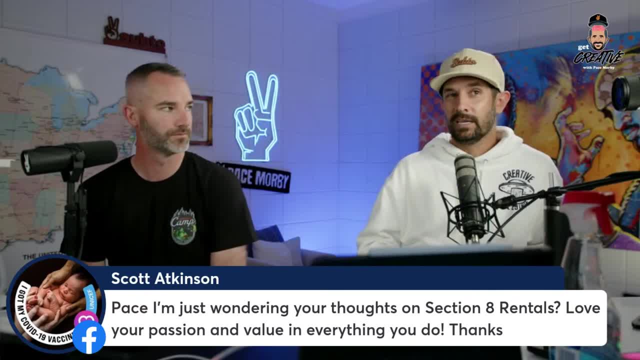 What I found is that section eight required me to buy in areas I did not want to own properties. Yeah, Sorry, High crime, High crime, Poverty, Yeah, A lot of poverty stuff. Um so I- and also here's the other thing about section eight- 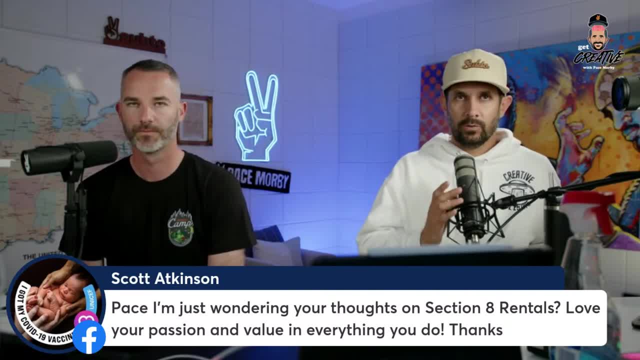 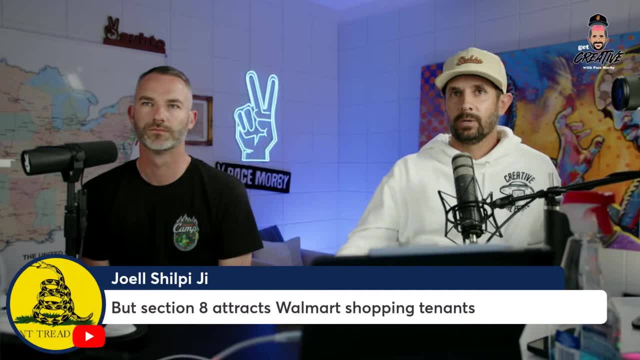 You're buying in an area that does not appreciate as fast as other areas that do not do section eight, And so it kind of depends on the game you're trying to play. Okay, There you go. Um, section eight attracts Walmart shopping tenants. I do shop at Walmart, just so you know, And when I shop at 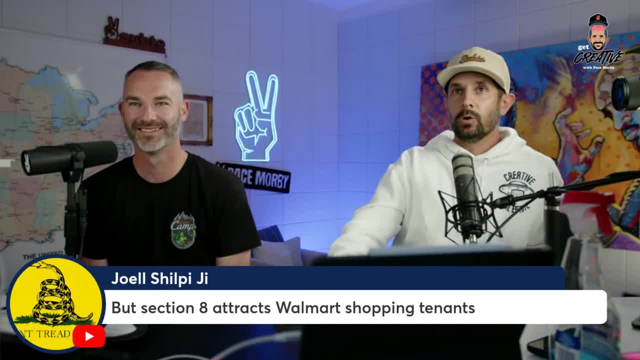 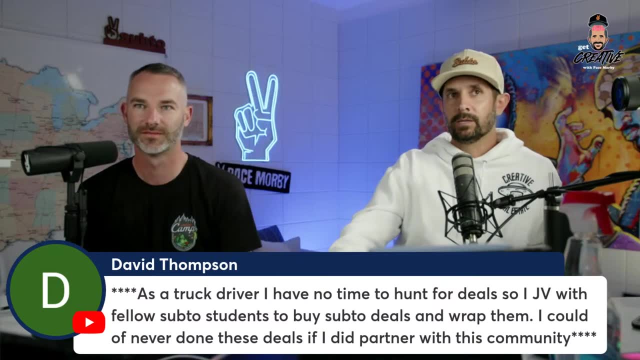 Walmart, I do wear my Crocs. Okay. So this is David Thompson says. as a truck driver, I have no time to hunt for deals, So I JV with fellow sub two students to buy sub two deals and wrap them. I could have never done any of. 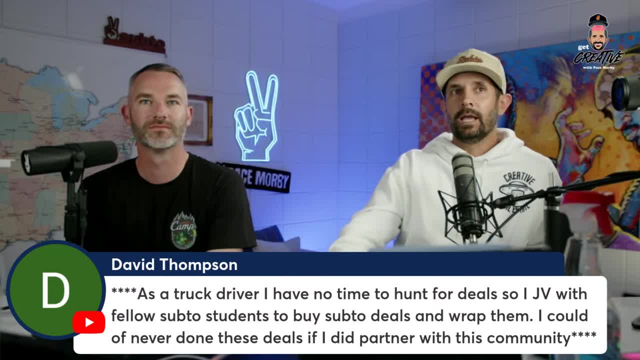 these deals. By the way, I saw David Thompson in Orlando the other day. never done any of these deals. If I did, if I did as I did when I partnered with this community, there you go. Love that brother. Thank you so much, So people really love. 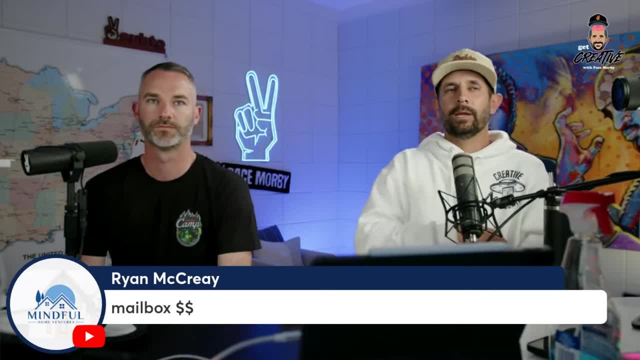 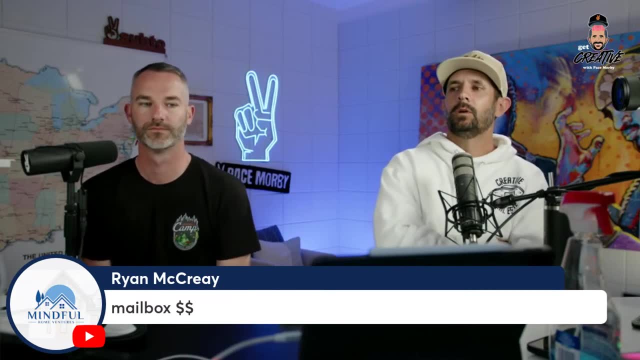 it's interesting to me, like section eight. people like it's guaranteed money. Okay, Let's take regular rentals, For example. what's the average default rate on a rent? Does anybody know that? I don't know the rate. This is what's so. 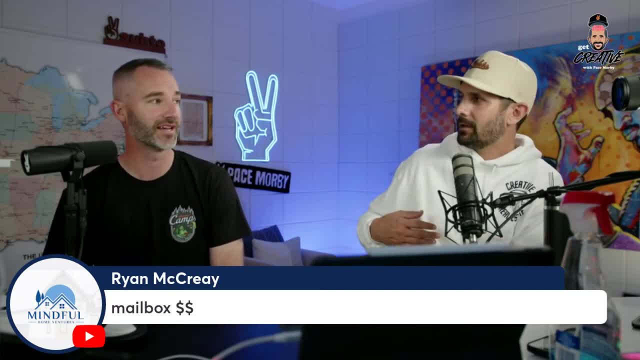 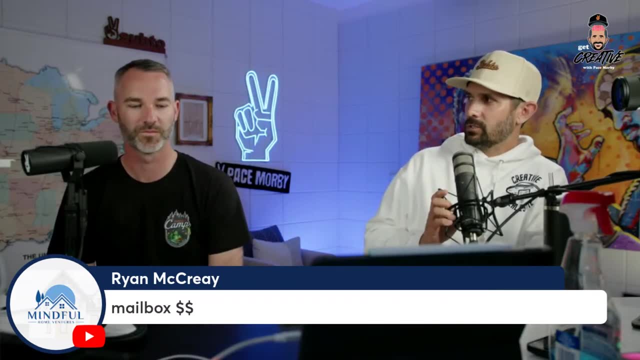 interesting to me about section eight. Most people don't know this- And is it like a similar rate? It's so small, Yeah, The amount of people that actually default on their rent versus section eight, which is like you do still get section eight. 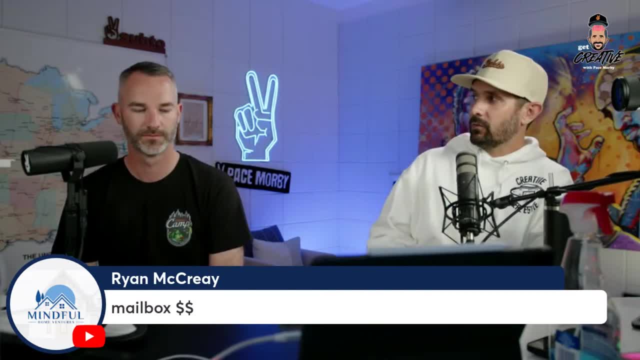 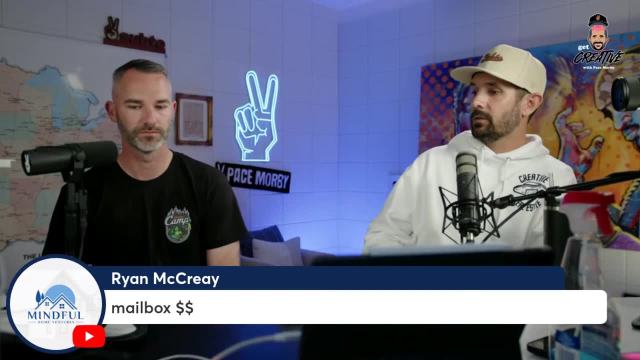 defaults. Yeah, Okay, The government is not paying their full rent. Do you know about that? No, the government does not pay their full rent. They, the government, subsidizes their rent, And so the tenant is actually paying something. So, just because the section eight, 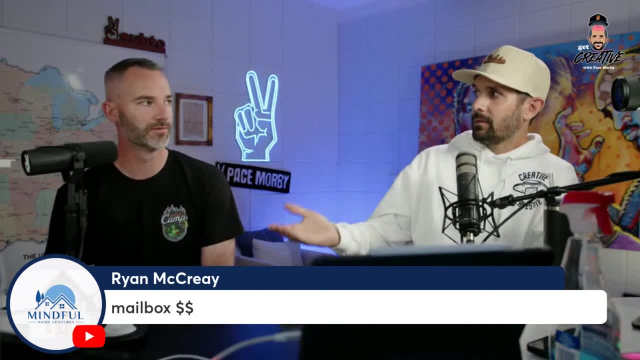 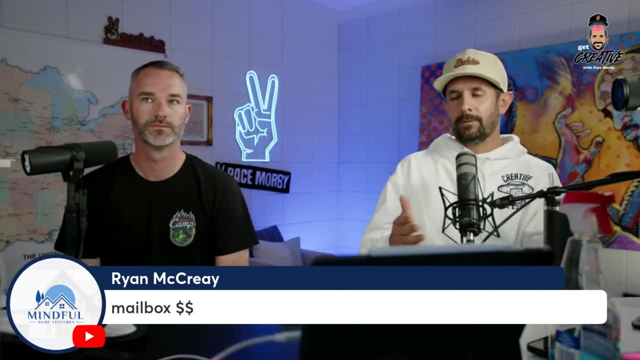 paid doesn't mean the tenant is going to responsible for a portion. There you go. They're responsible for three, four or 500 bucks right. Smaller amounts, Okay. so you're attracting a tenant, right That has to use government assistance. 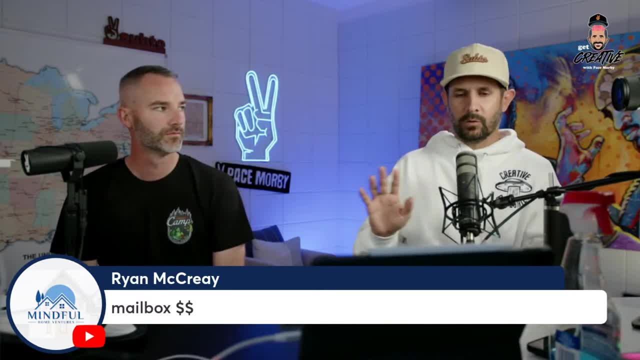 to rent there. Perfect Okay, got it, No problem. I love that. It's a great program. It's a great program. It's a great program. I said it three times. I don't want it to go away. However, 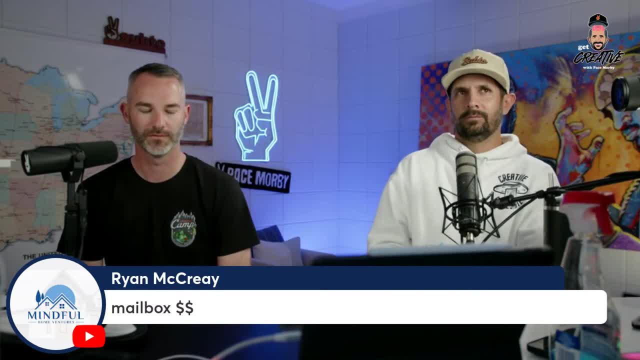 what is the default rate for regular rental? Is it 70% of people don't default. Is it 80% of people don't default? It's guys, it's over 90% of tenants do not default. So when you guys. 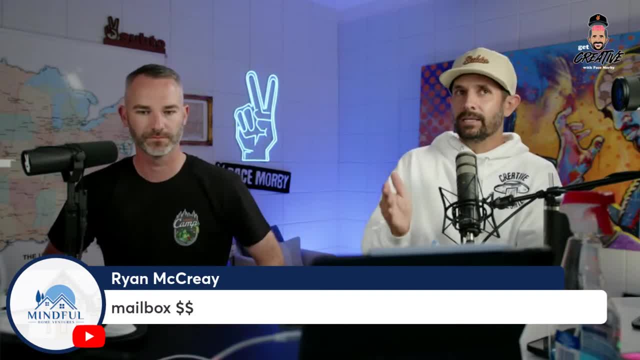 are chasing government cheese. I'm not saying it's not a good strategy. It's just that people get so excited about the section eight stuff right now because there's a guy out there that's in. he's like doing ads in front of a Bugatti And he's got a car. 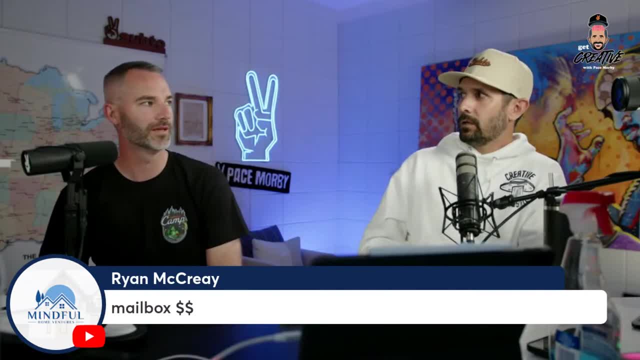 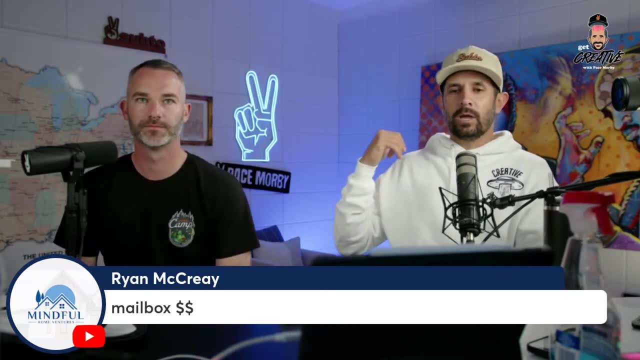 a garage full of like really fancy cars. Oh, I know, Yeah, He's not a bad guy. I'm not saying he's a bad guy, Yeah, Just his strategy. But his strategy is let me attract people that are like guaranteed money, Bugatti. Look at my beach house, Look at. 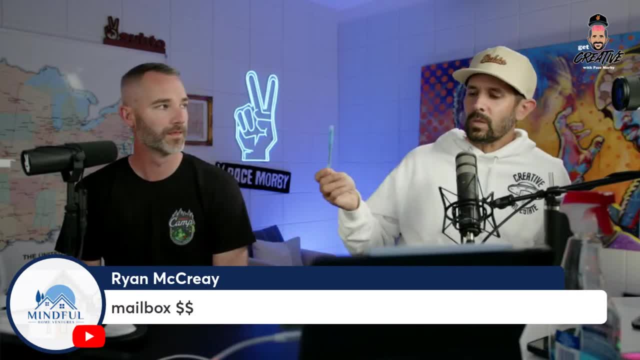 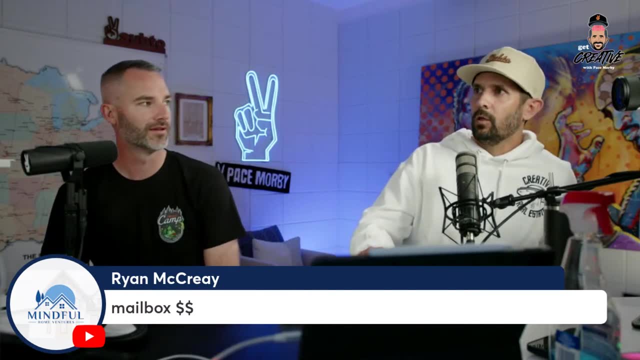 my this, And you know what they call it. It's lifestyle Ladies, And I can't remember the third L, But it's a Tai Lopez market. Yes, It's the three L's as they call it, So it's like lifestyle. 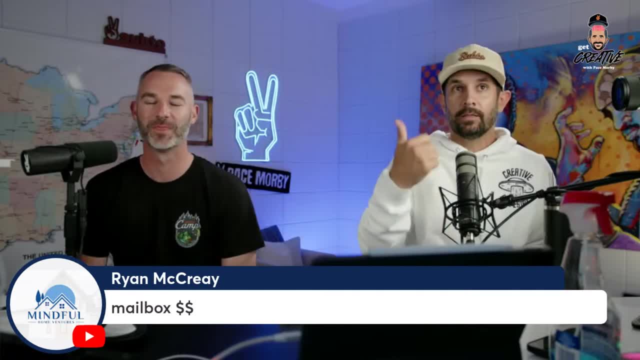 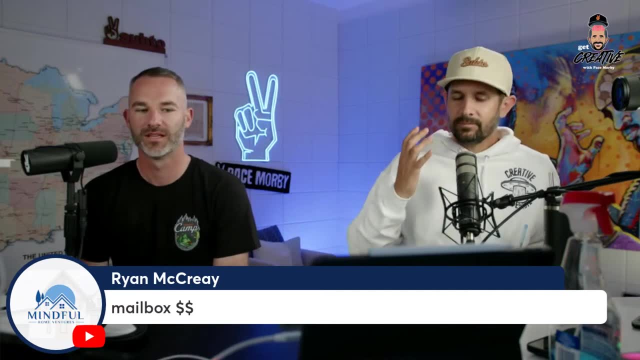 ladies and land, Oh, Lamborghinis, Lamborghinis, ladies and lifestyle. And when you see people that are marketing that way, guys Be careful. Okay, when you, when somebody has to do an ad in front of a Bugatti and has to do an ad in front of a mansion, 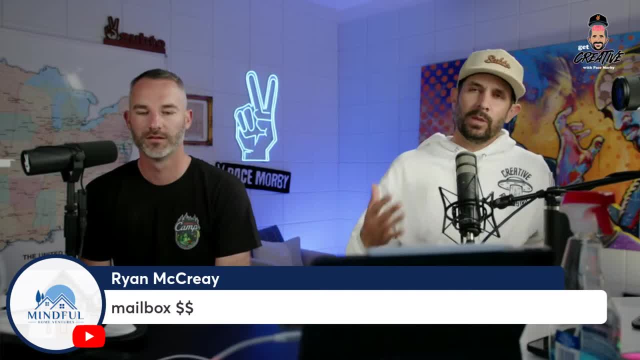 And like: this is my lifestyle, This is what I make. Just be careful. Doesn't mean that he's a bad guy, It's an attention grabber. But right, a red flag. Okay, just could be a red flag. 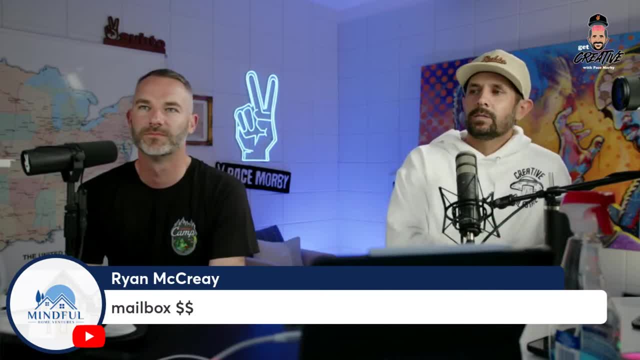 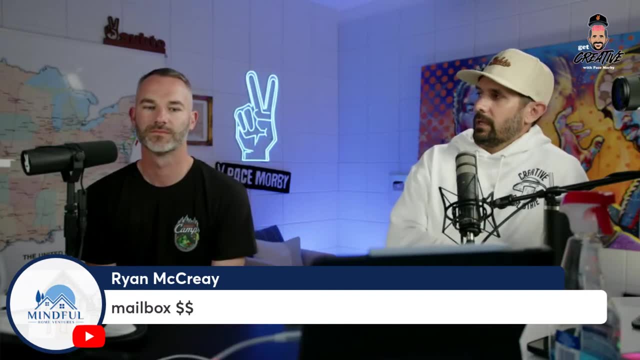 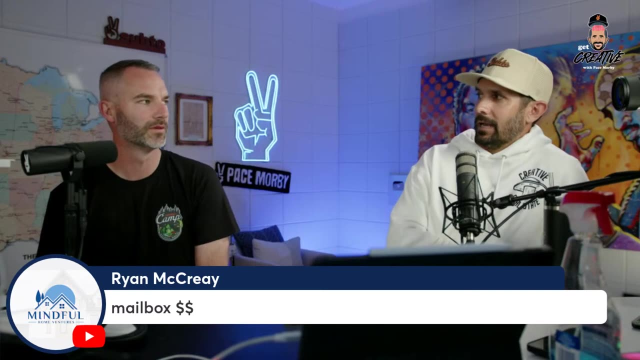 Lamborghinis, ladies and lifestyle. So I look at section eight And here's the challenge with section eight: If a section eight tenant doesn't pay their rent, can I evict them like a normal tenant? I don't think I cannot. They have rights that regular. 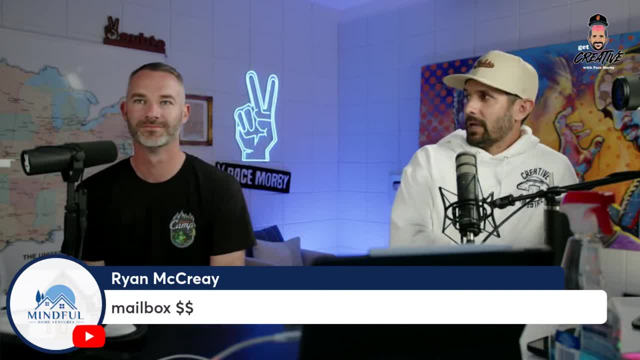 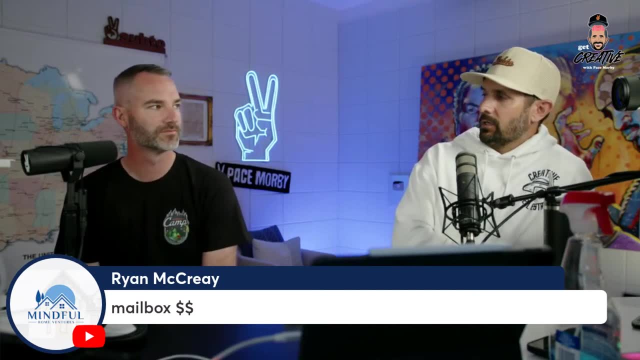 tenants do not have California style. California style And it's a government program. you sign off on this and you're not going to immediately kick them out. You have to go through this thing and arbitration and blah, blah, blah Like dude I'm not. 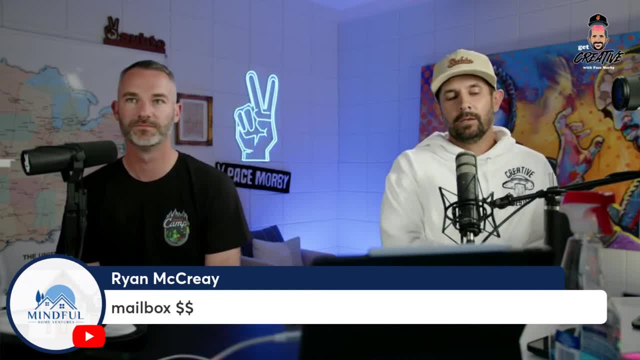 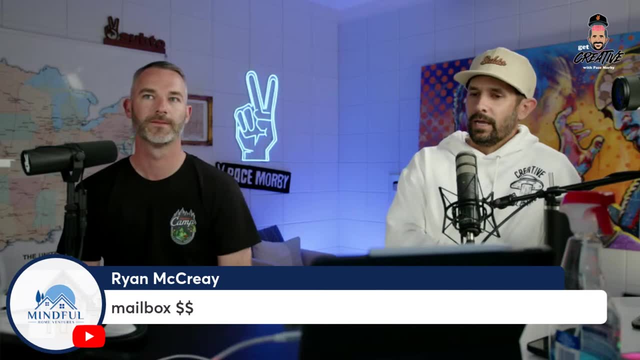 willing to do that. That's the headaches Yeah right, I had in my 43 unit in San Angelo, Texas. we had six people that were section eight tenants in my in my thing. they weren't paying. One guy was threatening one of our students- She actually, she was actually. 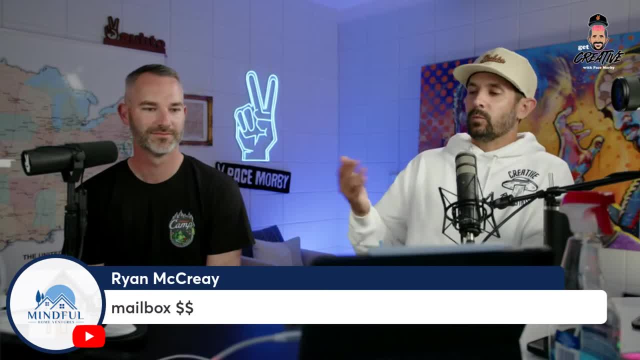 in the yearbook. I was just looking at her. She came with me. She's like: Hey, base, you're in San Angelo, Can I come hang out with you your units? I go, Yeah, come over and hang out, But I 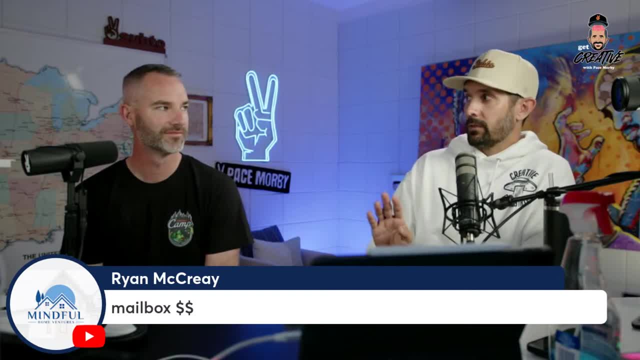 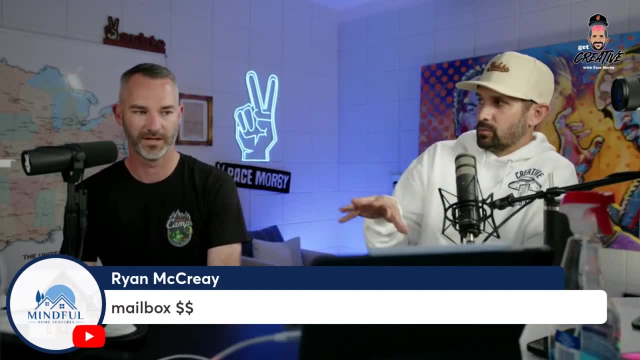 want to let you know I have six, 106 tenants that we're calling the police on. They're attacking other tenants. I just want to let you know that I've lost like 14 of my tenants because of these six people, So just be careful She comes over This. 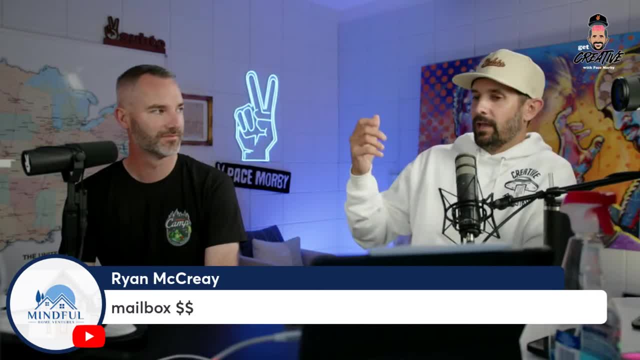 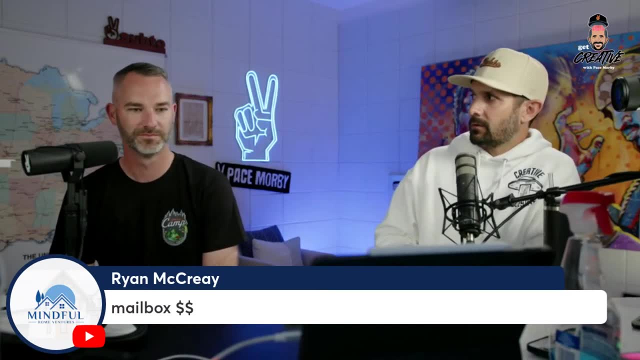 guy has his cane out, He's attacking her And we have to get the. we have to get three people around her to get her into a car to get her off the property. That's it. That's a section eight tenant. Okay, It's like live world star. It literally was like live world. 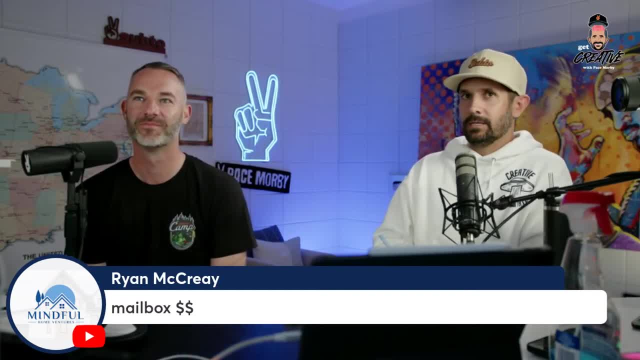 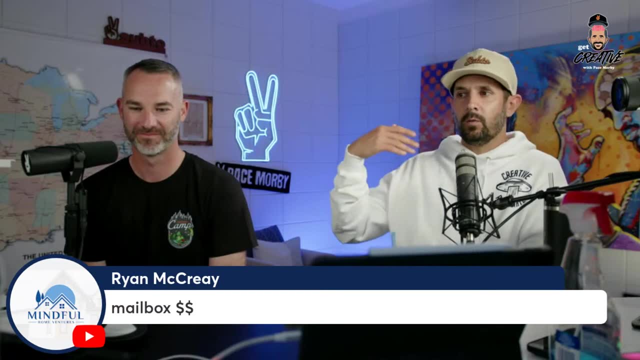 star, We actually put it on the YouTube channel. It's a phenomenal video. if you guys want to see my tenant attacking one of my students, So that's section eight. Yeah For me. when people I go, I want that mailbox money, I want passive income. 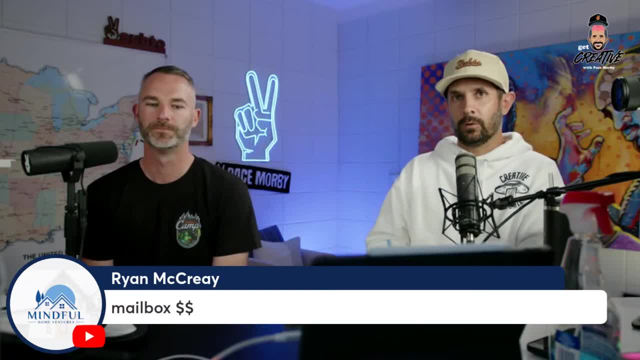 guys. Section eight: money is not passive income. You're dealing with tenant issues frequently, Mm hmm, Here's the other thing about section eight: tenants Do they treat the properties better or worse than a regular tenant that does not need government assistance? What do you think? 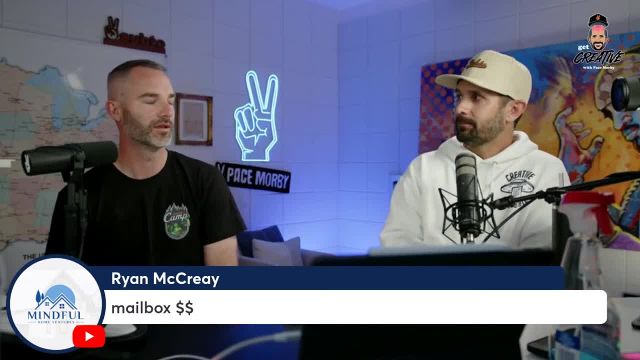 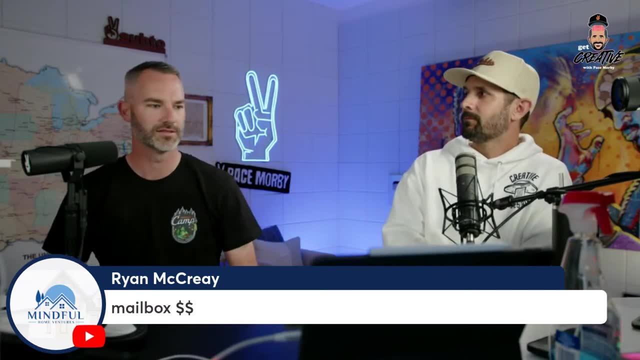 Oh, I was reading the next question, Okay. so tenant quality: right Yeah, If I have a tenant that section eight versus a tenant that's not section eight, which tenant do you think is going to treat my property better? Oh yeah, non section, non section. Yeah, they're more. 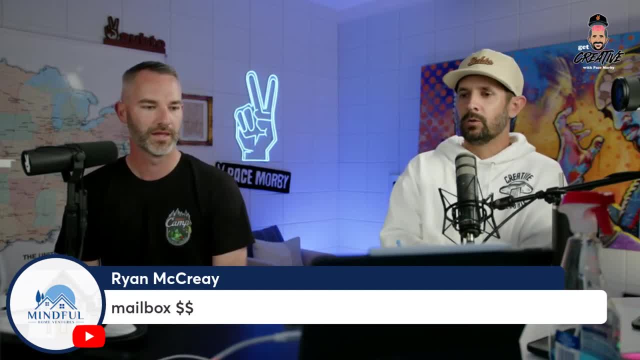 responsible. They're way more responsible. They didn't need government assistance, So they have to be accountable And people go. Well, here's the thing: pace. If they damage your property, they could lose their section eight entitlement. Yeah, do you think that's stopped them from ruining their life so far? 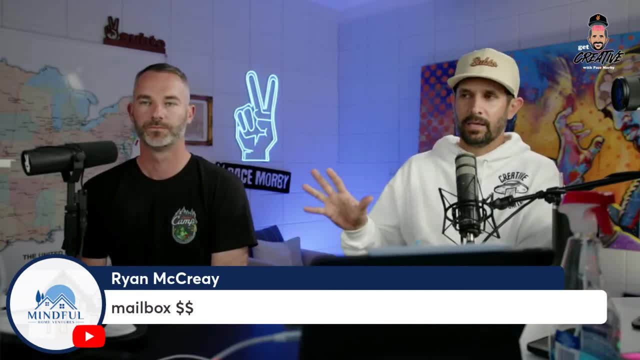 Now, not everybody that's on section eight has made bad decisions. I get that. I made, I made a generalized statement, Totally get that. But I want to let you know that the overwhelming majority of section eight tenants leave my properties in $10,000 more damage than a non section eight. 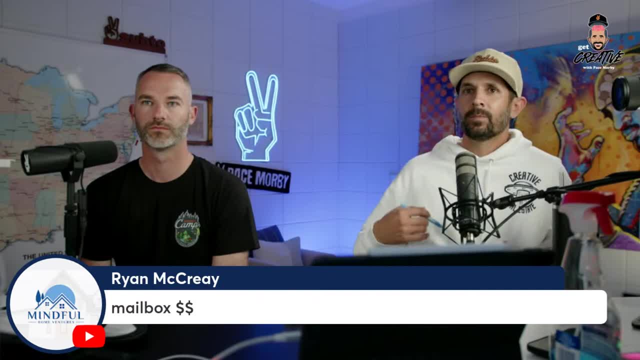 tenant. So when people go well, section eight pays a little bit more money. See, Israel is always somebody that's like: Nope, not true. You have two tenants, Okay, Israel Miller. Miller has two tenants that are section eight, people that do everything guys. 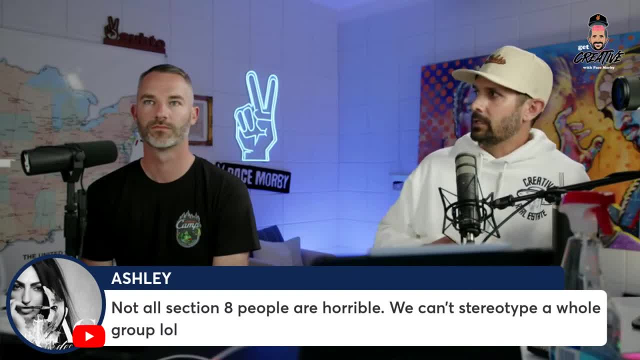 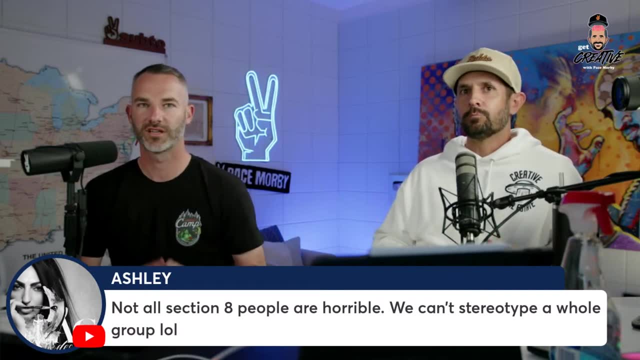 See the same thing, Ashley, I already said this. Did I not hedge this? Did I not say I'm not talking about ahead of it? I tried to get ahead of it Always, always, always, guys more. just the comparison to normal renters. I'm comparing it, Look. 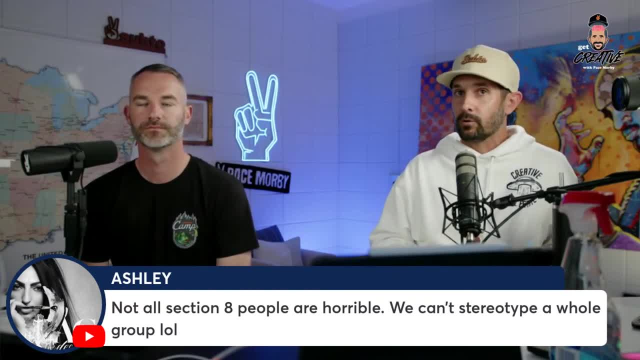 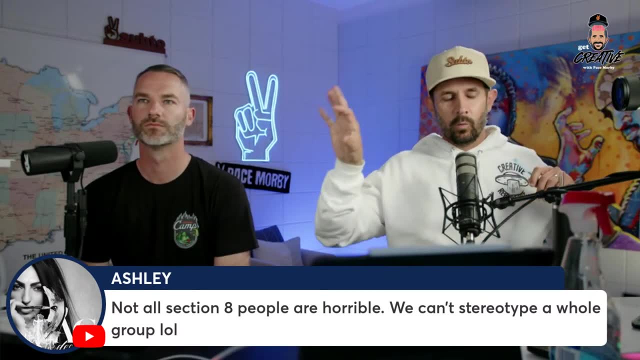 there's amazing sex section, eight tenants, just like there's horrible regular tenants. Okay, That in some situations. but if you over, if you generalize it and you take the worst of both sides and the best of both sides out of the equation and take the middle, the overwhelming- 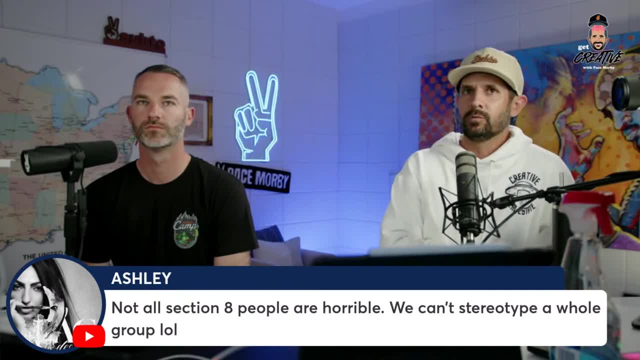 majority of my section eight properties have $10,000 more of damage on a property when they move out than a regular tenant. So when people say, Oh, section eight pays more money, guys, I have 2000 doors, 2000 doors, I have 2000 doors in my portfolio. 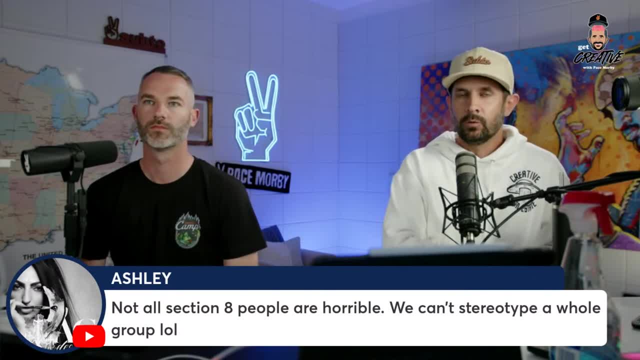 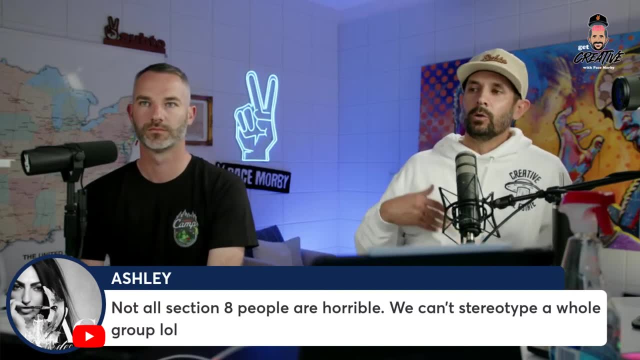 Okay, I'm going to say that again. I have 2000 doors in my portfolio Doesn't mean I know everything. No, I do have some experience if I have 2000 doors. So when you're looking at those deals and 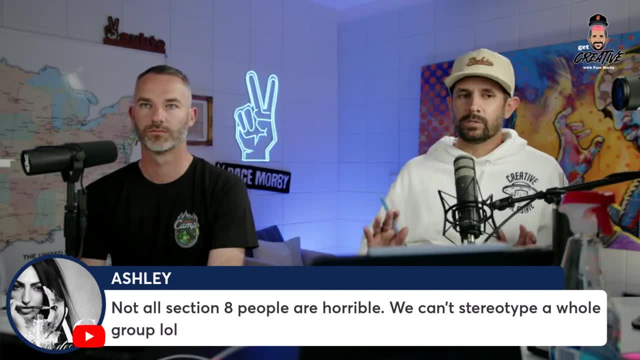 you're saying: I really want to go section eight. here's the challenge with section eight. The biggest challenge with section eight is that there you can't just go and pick any house and turn into a section eight house. You can't, You have to go. 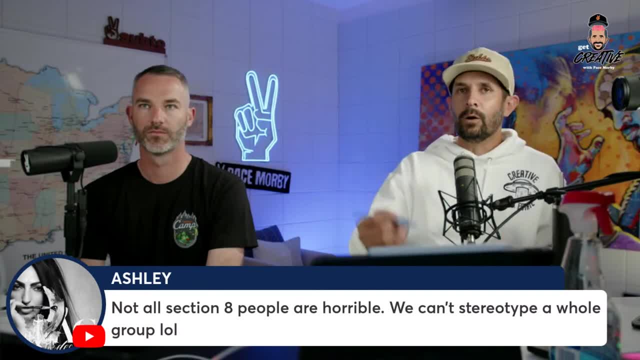 and find areas and sections where they have vouchers. I have bought houses. when they say: Oh, vouchers are available, I go find a house, I buy the house And then I go and I go: Hey, I need a voucher. They don't approve. 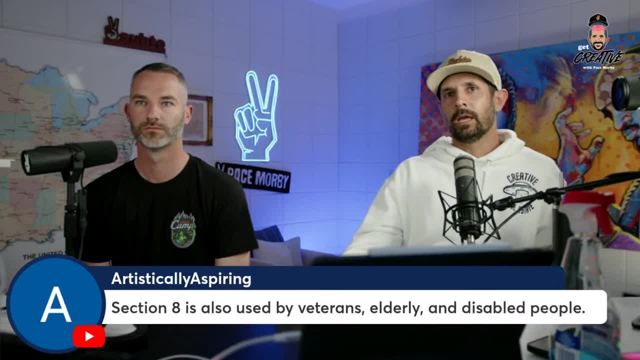 the house. Okay, Okay, Got it. So there's all, guys. I said this artistically, aspiring. I said this about 17 minutes ago. People choose to listen to what they want and not listen to what they don't want. I said, guys, there's amazing, section eight. 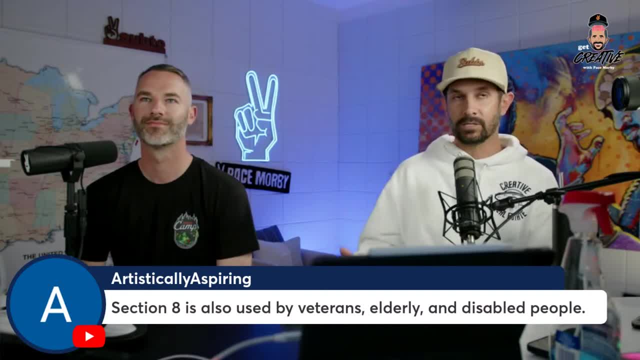 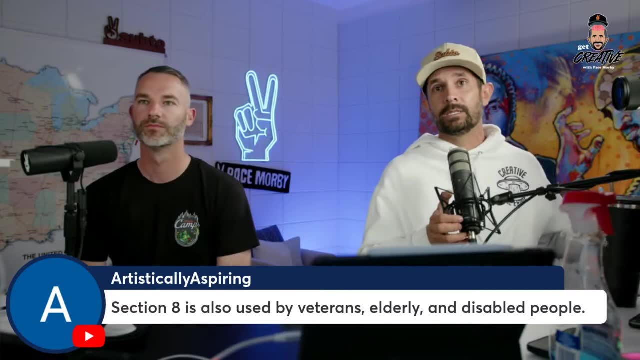 tenants. There's a lot of people that use it, that are not bad decision makers. They didn't do it something poor. I made that statement. I made it so clear. I just said it now a second time. Okay, I just made it a second time. I now I'm going to make it a third time. so 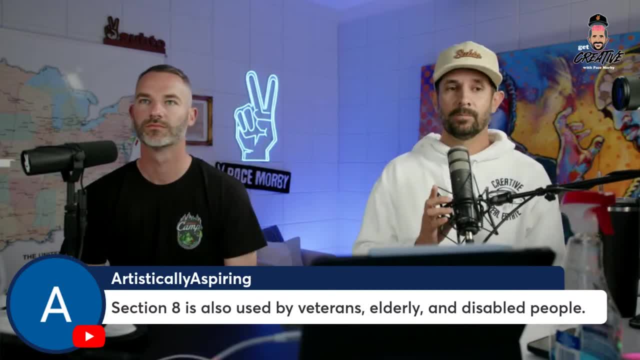 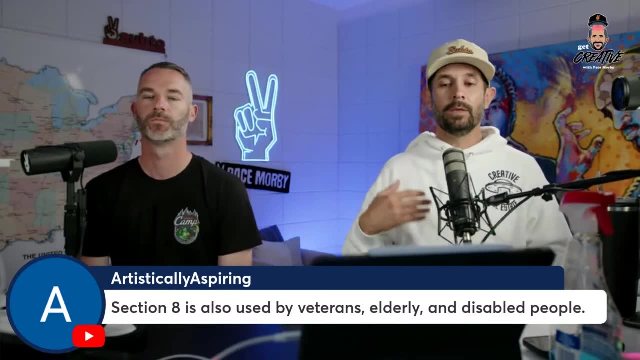 we can move past this. Okay, Section eight: tenants. There's a lot of them that are amazing. A lot of them are amazing and they did not make bad decisions. Maybe they were dealt a bad hand, Maybe they're veterans that just are out of work, or 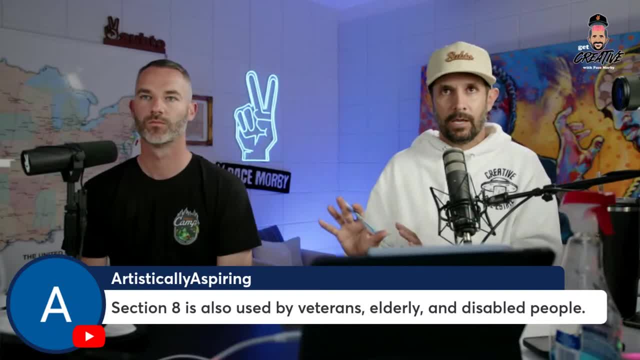 they're injured or whatever the heck. I get all of that. Okay, I get all of that. Thank you so much, for we've made that comment five different times now. Okay, Now let's move on and just talk about the facts. If you have 20 regular rentals, 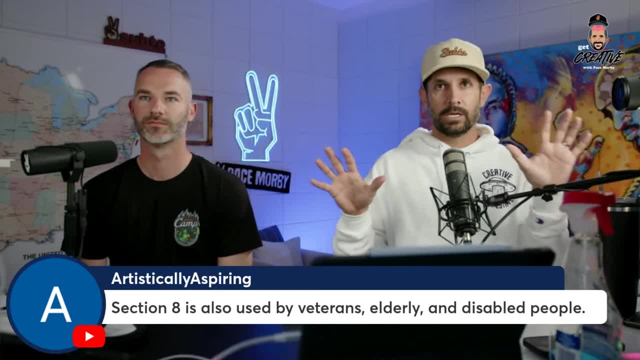 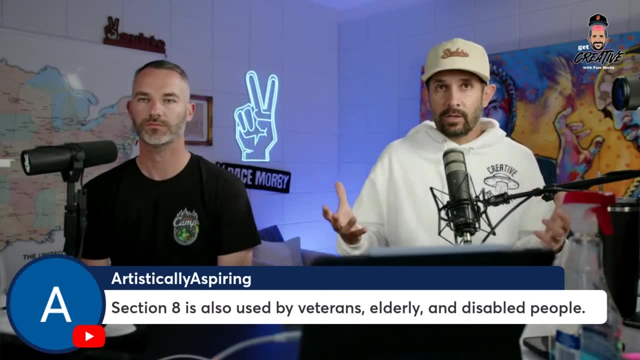 and 20, section eight rentals. you are getting way more damage on your section eight tenants. You are getting just as much default rate on your section eight as you are in your regular tenants. That's all I'm saying. So when people make the 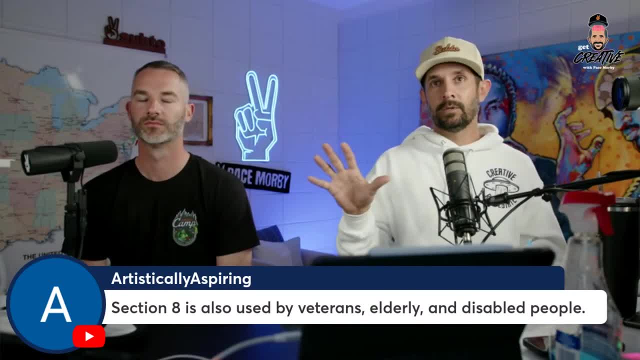 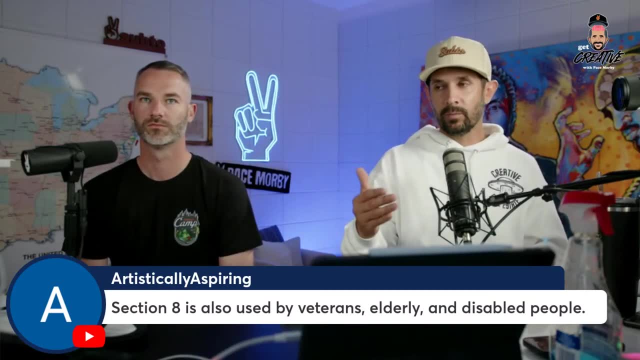 argument: section eight has guaranteed rent. No, it does not. Section eight does not have guaranteed rent. You do get a portion of it that is guaranteed from the regular tenant, from the government. but when your tenant does not make their portion, that part is not guaranteed. Cool Got it Does. 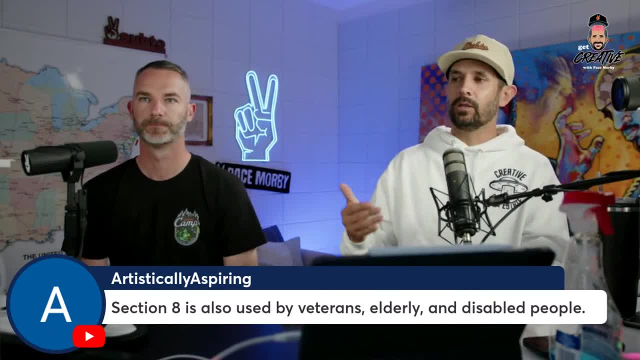 section eight pay you a little bit more money than a regular tenant can? Yes. However, when you take consideration into the amount of damage that comes from a section eight tenant over, let's say, a four-year time span- four years, $10,000 of damage. 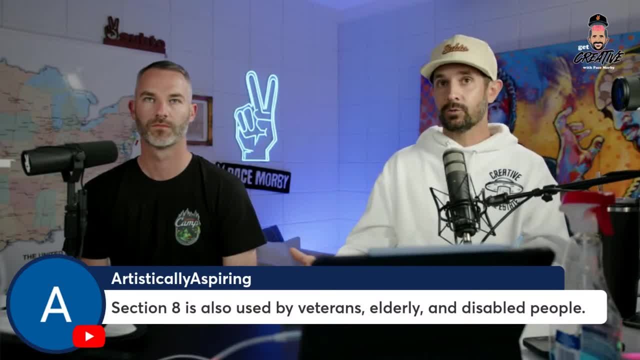 that's $2,500 of damage per year extra. that's being put on the. that's what? $200 extra per month. It waves and wipes out the extra cashflow that you're getting from the section eight tenants. So I disagree. from my own personal experience that section. 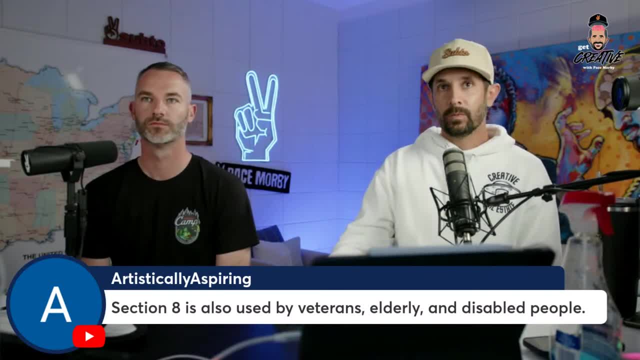 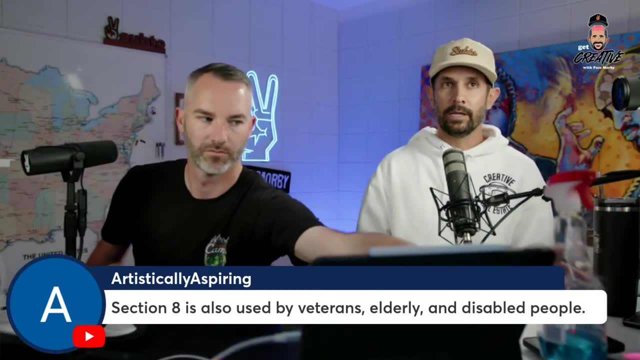 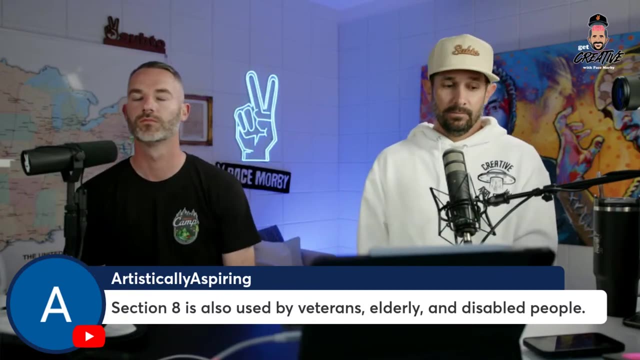 eight pays more money. Okay, There you go. Now does sec. is section eight Awesome? In a lot of ways, Yes. However, when you go and you do section eight, what are you running into? You're running into areas that are a little bit less amazing, And let's say that I did make the 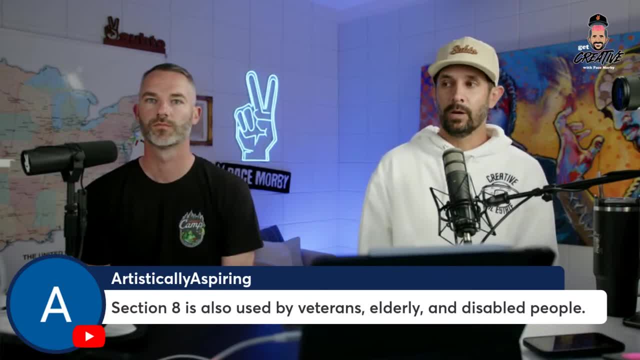 decision that I wanted to convert my property into a midterm rental, or I want to convert my property into an Airbnb or you know um mental wellness house or something else- a different exit strategy. You can't just do that in a property that you bought for $60,000 in Ohio in the middle. 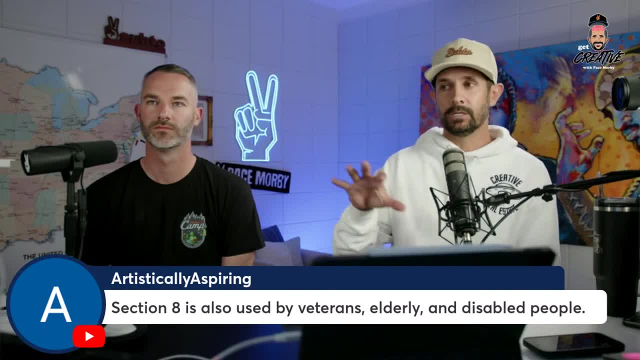 of nowhere. Most of the people that are doing section eight are buying a property that's in the hood, that nobody wants. They do not appreciate if they're $60,000.. Think about this If they're 60 to $80,000 today, when real estate is at an all time high. I'm going to teach you. 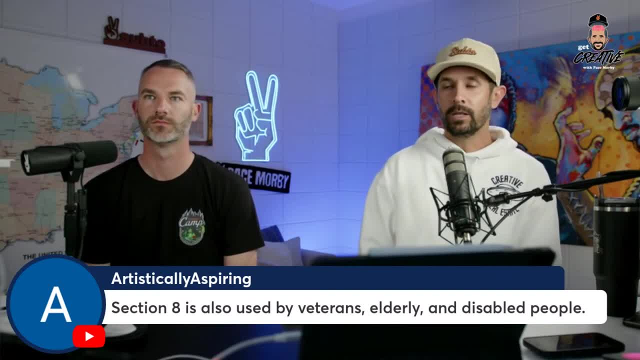 guys something about real estate. You should all write this down. Nobody makes money from cashflow. This has been talked about on bigger pockets. This has been talked about on my show. Nobody makes money from cashflow. Where do you make all your money? 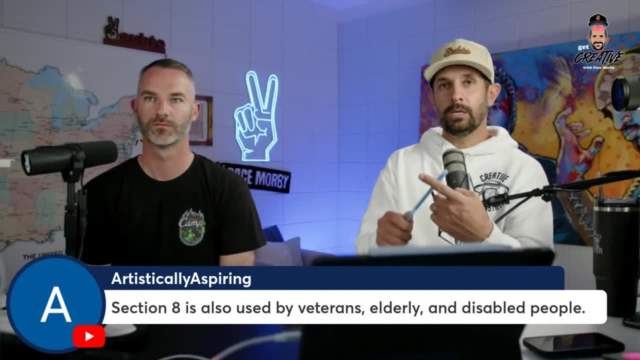 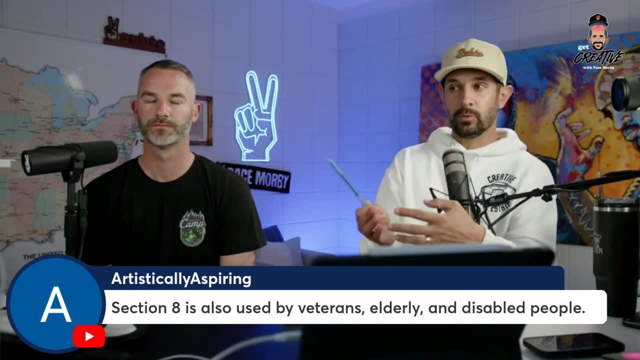 You make money from cashflow. You make money from cashflow. You make money from cashflow. You make your real, significant money in the tax savings of real estate. That's massive, Okay, The other thing and, by the way, if you're buying $80,000 properties and you're actually putting 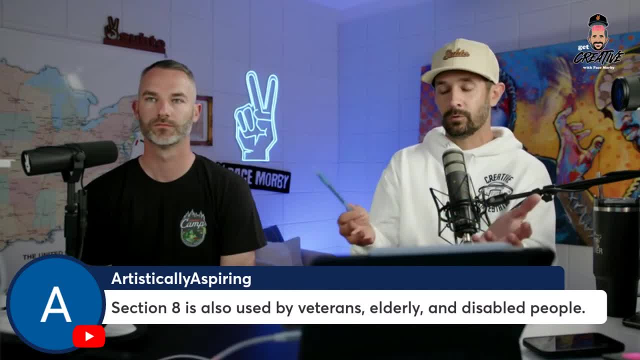 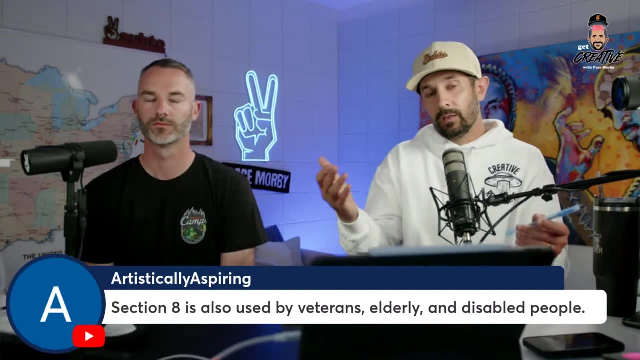 30% down and getting seven or 8% interest loans, which is what people are doing in section eight. you're missing out. Your set your tax advantage is only $80,000 versus. I can go do a sub two deal in a good neighborhood at $250,000 with less than 5% down and get a 3% interest rate deal. And I can turn that into a regular rental in a market That's going to appreciate. which property is going to appreciate more? The one that you bought for $80,000 in 2024, the property that you bought for $250,000 in 2024.. What's the likelihood that? 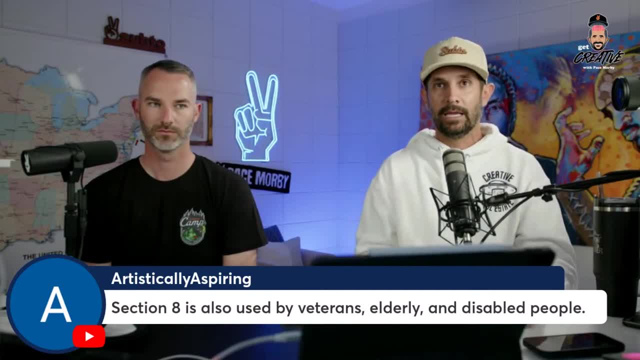 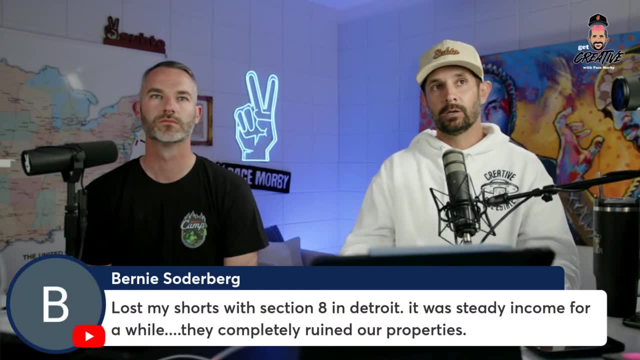 this two, 50 is going to be out, surpassed by the 80, impossible, impossible. Okay, There you go. Bernie Soderbergh says lost my shorts with section eight in Detroit. It was steady income for a while and they completely ruined our properties. Now is that every? 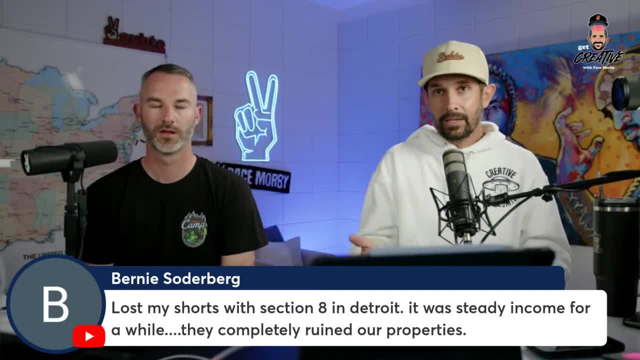 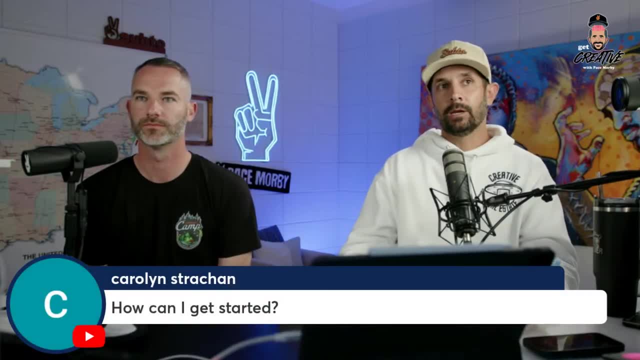 every tenant? No, And Bernie's not saying that is every tenant either. Just being aware of it, Just an investor doing your due diligence. There you go, That's it. That's all we're talking about. Well, now Carolyn says: how can I get started? Carolyn, let me show you something that's pretty. 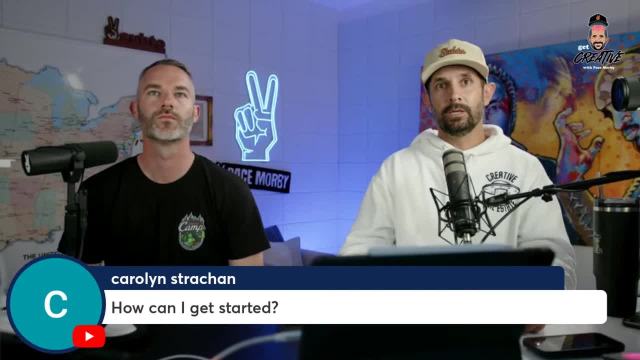 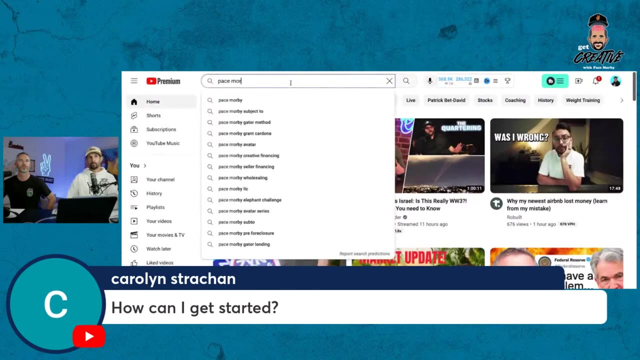 helpful: Watch, watch this. This is really really cool. I will give you something that's super helpful If we go to YouTube and we type in. one of my favorite things to do on YouTube is this: check this out. Type in pace Morby. 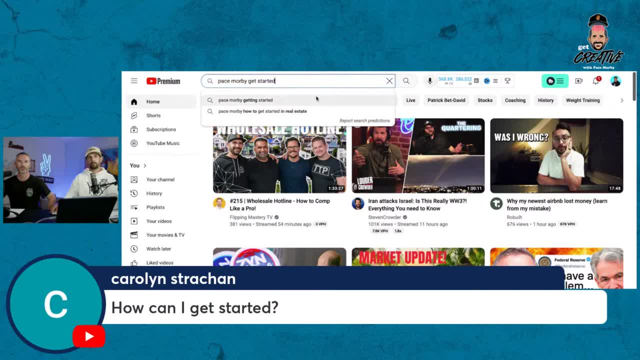 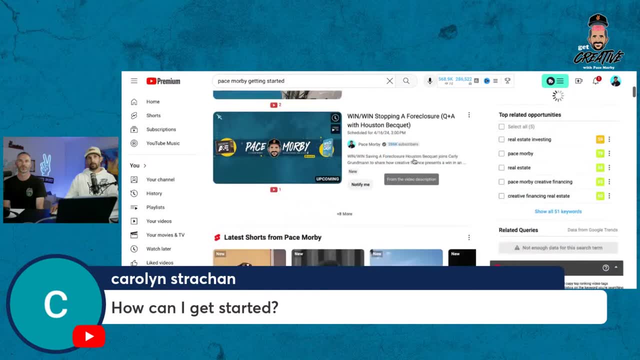 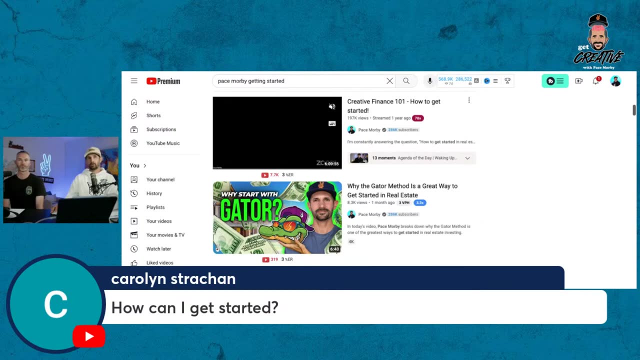 Get started. Getting started step-by-step in 2024.. How to- okay, Let's see, I know I have one more. Okay, Creative finance 101.. How to get started: 197,000 views streamed a year ago. Okay, That was also a. 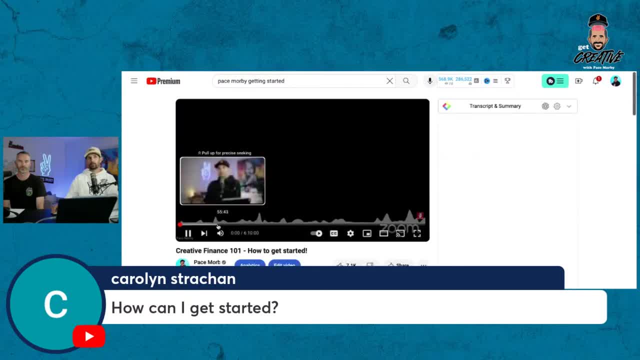 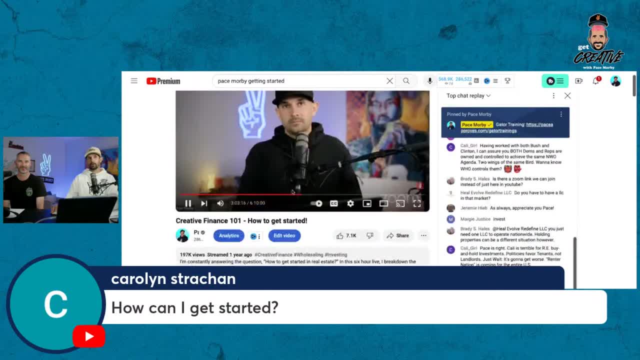 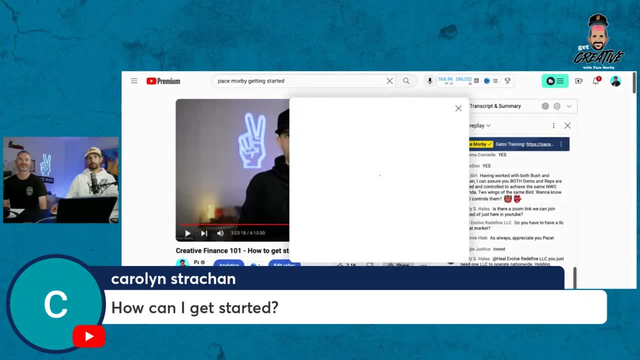 six hours. This is also a year ago. Apparently, that's a question for Nancy, growing my beard back then. So there you go, Get how to get started. Let me give you. I'll share this video for you and go and watch that video. That's like a little masterclass. all for free for you, Nancy. 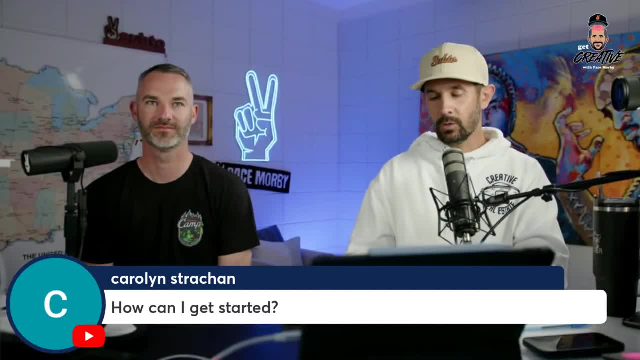 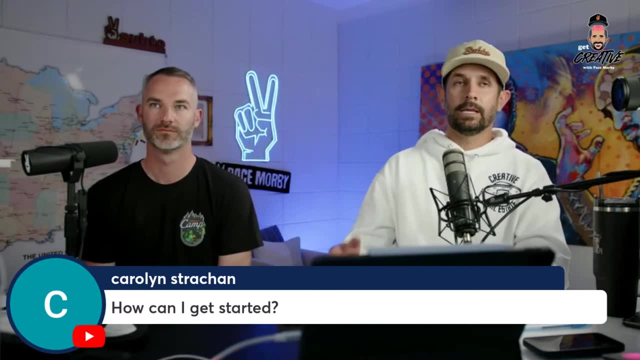 should help you out quite a bit. And so again, when you guys are having conversations about: Hey, how do I make money in real estate? Cashflow is great, but what cashflow really does is it helps you manage your vacancy, It helps you manage your future repairs? 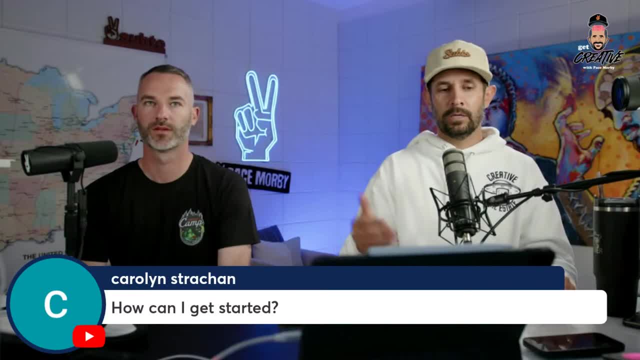 Cashflow might pay some bills and help you reinvest that money into future things. But really the biggest money that I make and everybody else I know makes in real estate is when you get your tax benefits, when your tenants pay down the mortgage. and biggest one: 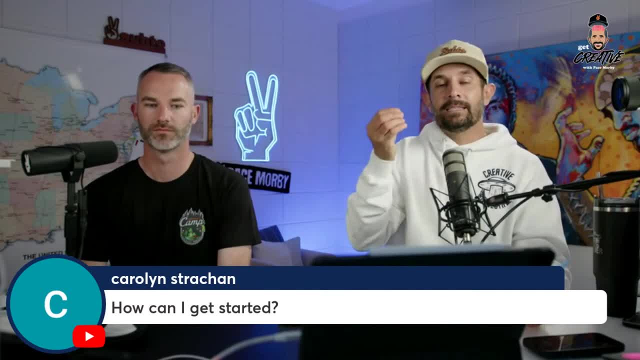 is when the property appreciates and you refinance that money out and you get that money tax-free. That's where the big, massive chunks of money come from. I did a D, I did a video, Um, and I'll explain this one for you guys in a second. but I did a video. 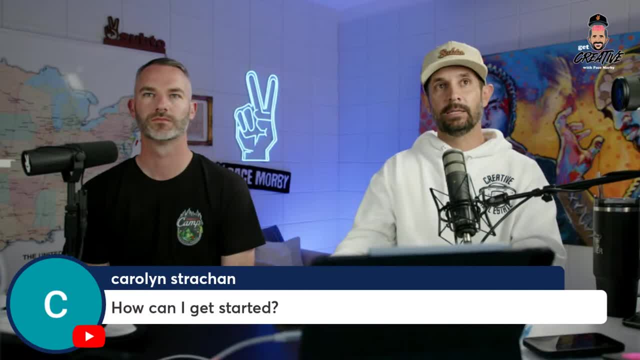 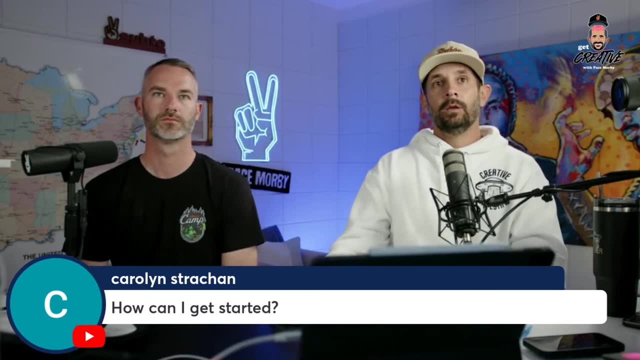 With um Jerry Norton up in Montana breaking down one of his deals- Let me see if I can find this face- Morby Jerry Norton. Okay, Um, dang, these are good. Him and I have done some good videos together. Jerry and I have done some freaking great videos together. Um, I have a. 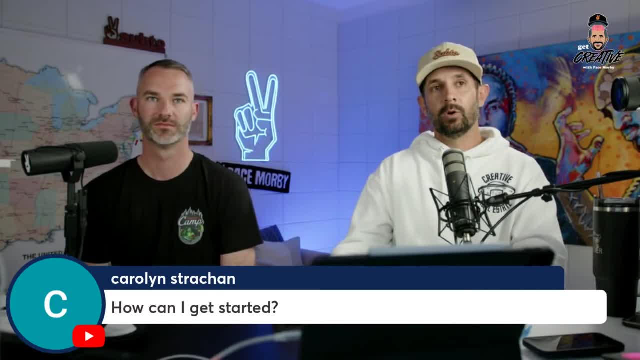 video that I broke down a property. how to find deals daily? Nope, not that one. There it is, Boom. I knew I knew I could find it. Here we go, guys, Let me show this to you. This is a great video because what it does is. it highlights that the majority of the 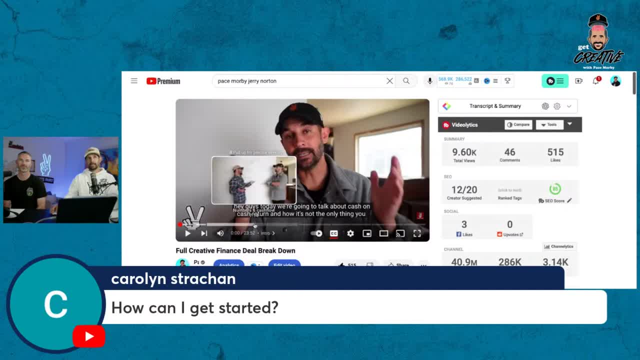 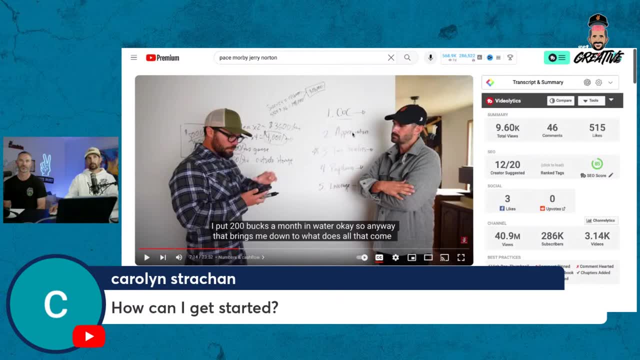 money you make over a five-year period on a piece of real estate is actually not the cashflow. And we go through, we break this down one by one. So number one is cash on cash return. Number two is appreciation, Three is tax benefits, Four is pay down, Five is leverage. And you look at the it's a mess. That's what you'll see. But the total return on this property in five years is $410,000. And the cash on cash return is actually the least amount of it. The appreciation is $225,000.. The tax benefits and the pay down are more significant than all of the cash on cash return. 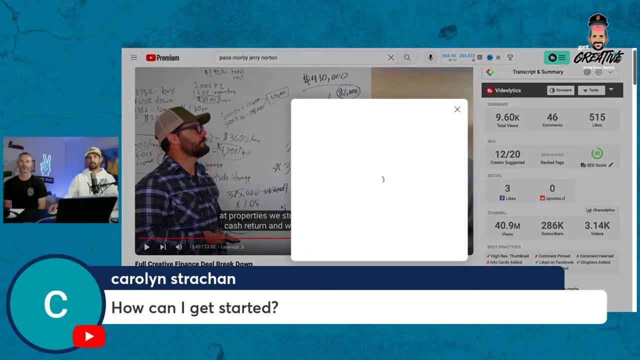 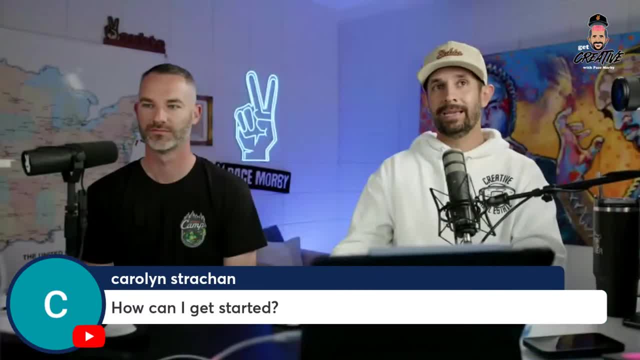 going to get out of it. You're not going to get out of it. You're not going to get out of it. So I realize I'm not making the money I need to make, which is the appreciation If you buy it. 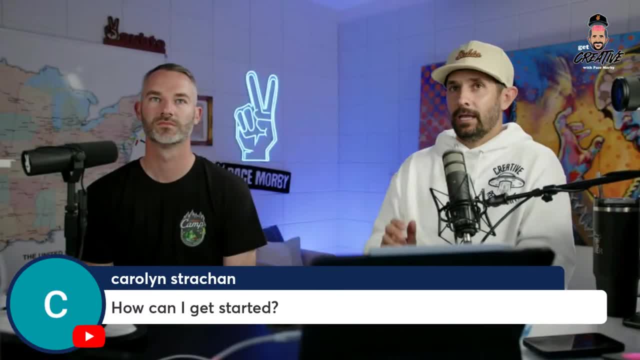 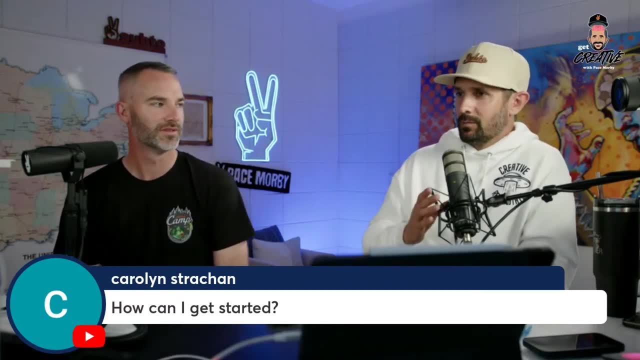 think about it again. If you buy a property today that is worth 80 grand in 2024, versus one worth $250,000, which one is going to be worth another $250,000 in 10 years, It's a no-brainer, right. 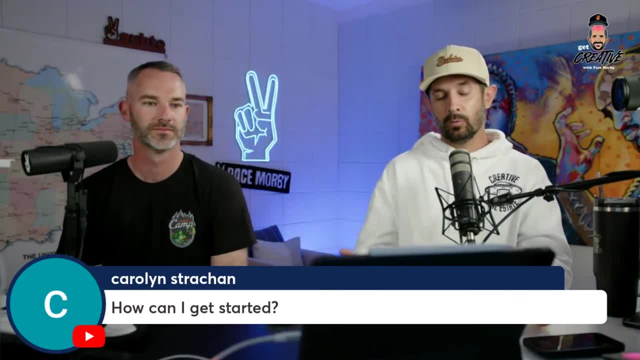 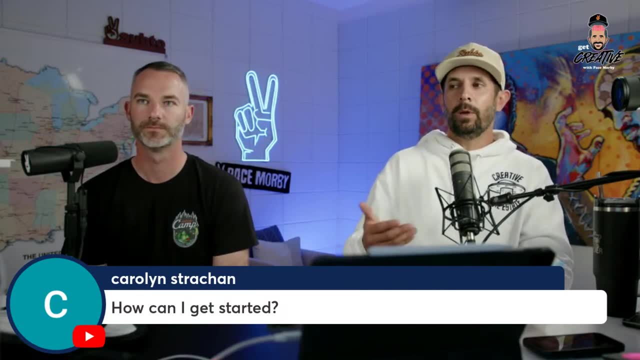 So by the and the other thing is you're buying an $80,000 property and you're putting 30% down and getting a seven and a half percent rate mortgage. right now with rates, It doesn't make sense. Well, Pace, why do I have to do that? 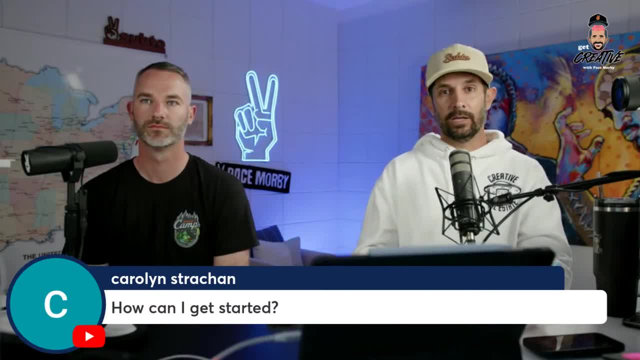 Well, because Section 8 is relegated to specific areas. Every county has different vouchers. You can't just go and go. I'm going to buy that house on the MLS and turn it into Section 8.. That is not how this works. 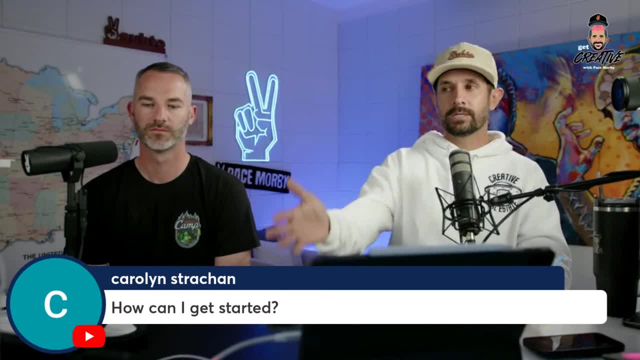 You have to go to specific areas that the government is willing to give vouchers for Section 8.. And if you're going into those areas, you're not always likely to find a property that you can buy sub to or seller finance. I personally would rather find a sub to or seller finance deal and then determine my 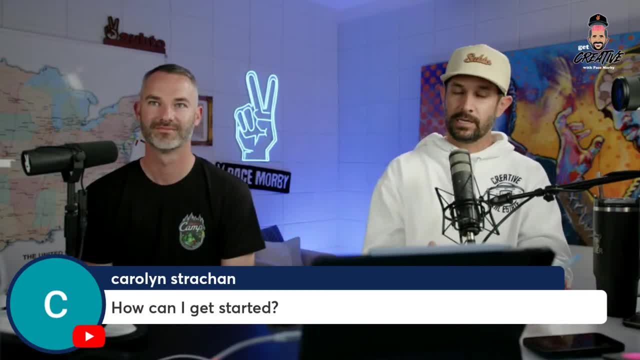 exit strategy because I bought it for 5% down with a 3% interest rate, knowing that I got a better deal in a good area, And I would then choose my exit strategy. Guys, if you're going after only Section 8 and you want to help people and you want to, 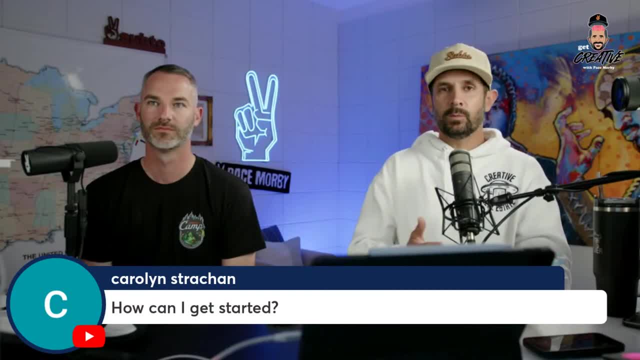 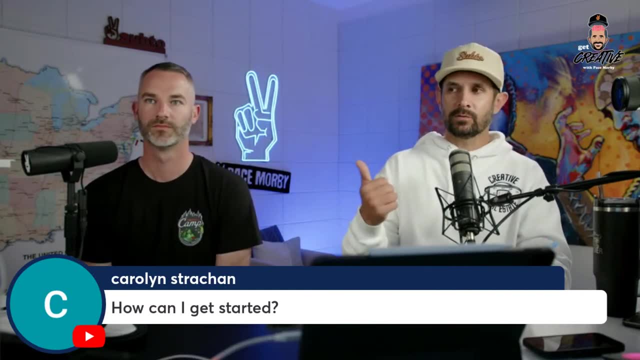 go after affordability. do pad split. Pad split is going to make you way more money And I would research pad split over Section 8 all freaking day long. More cash flow, less restrictions. I don't have to ask the government to pay me. 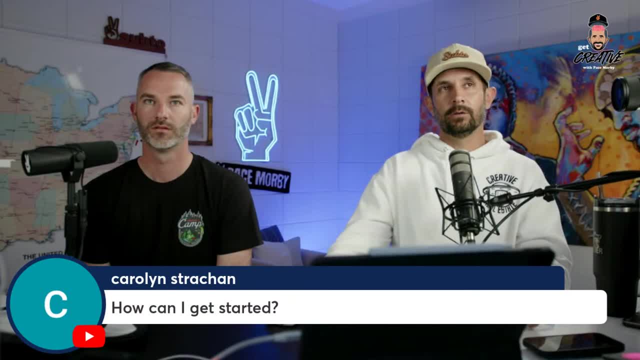 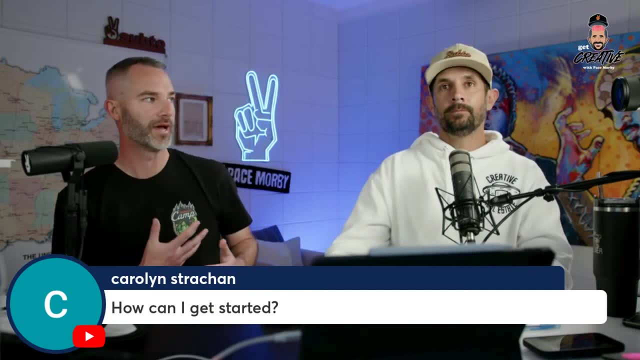 And I've got a property. I just did a breakdown of it on let's see here, Let's do another YouTube video. I'll give you guys this link in the side chat: Co-living. Well, the cool thing with that too, with pad split, is that the tenants are kind of accountable. 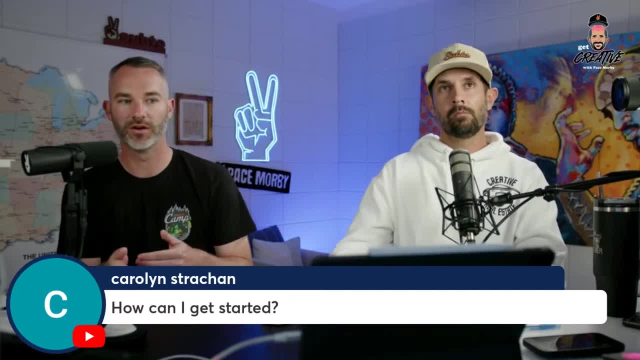 to each other. It's like they can do reviews on each other if one of them isn't holding up their end, And so there's that. Okay, let's go. Pace Morby pad split in YouTube. I have a really good one. 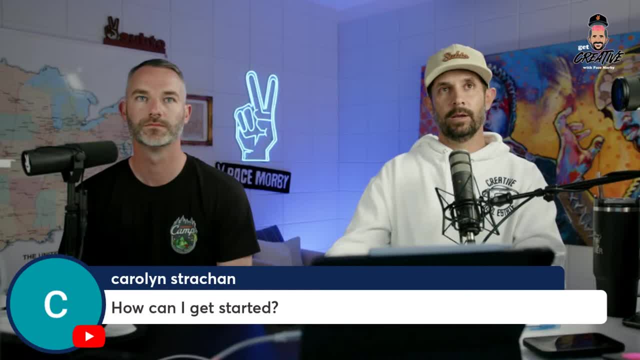 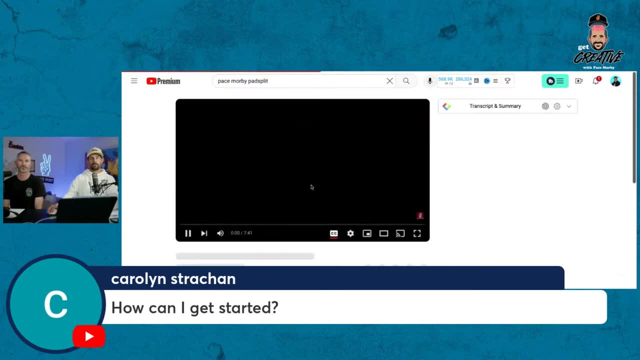 I think we just recently posted. It's a deal that I bought- No money out of my pocket, 2% interest rate. Already had five bedrooms in the deal. Oh, right here One month ago. Okay, use pads. Hey guys, how can you get this property right here? 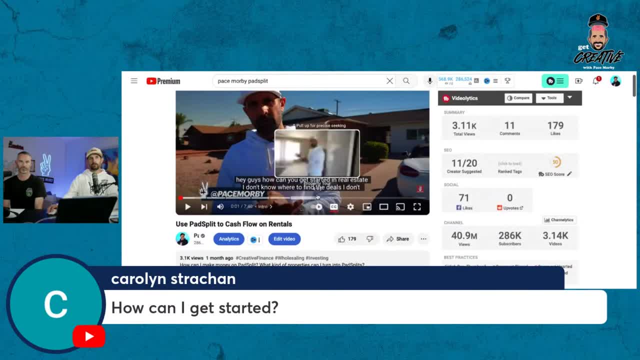 It's a seven minute video. We break it down on walking through the house. We show you exactly what it looks like. I did not do a dollar of renovation on this freaking thing. I bought it from a sub two student Right here, Luciano. let's see what the rate was: three to five. 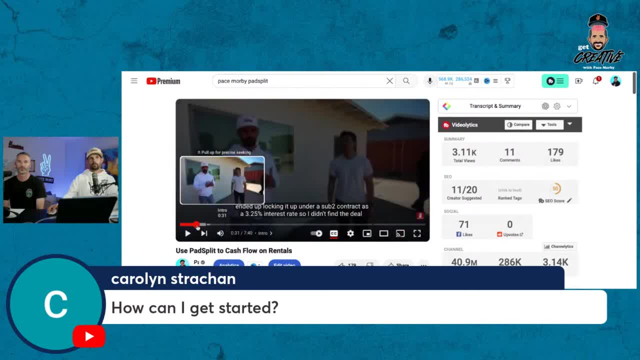 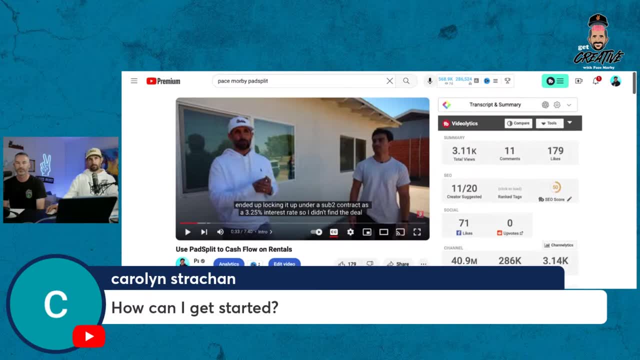 Okay, three to five, not not 2%, not 2.75, 3.25.. This was a month ago, So what would you rather do? Buy a gorgeous house in a wonderful neighborhood, across the street from a park, using pad split. with no credit check, very little down payment. I think I gave him 19 grand, but it came from a private money lender. Guess what I can't do when I'm doing section eight and I'm buying through a bank, I can't borrow money from a private money lender. 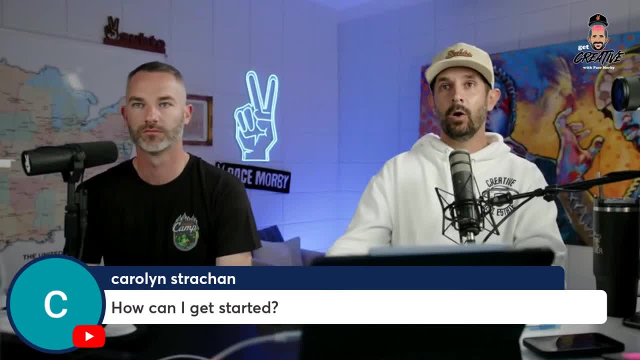 I have to have seasoned funds. That's like the amount of money that I have in my pocket. I would not. if I were you guys, I would not use. I would not. I would use section eight as one of my own. 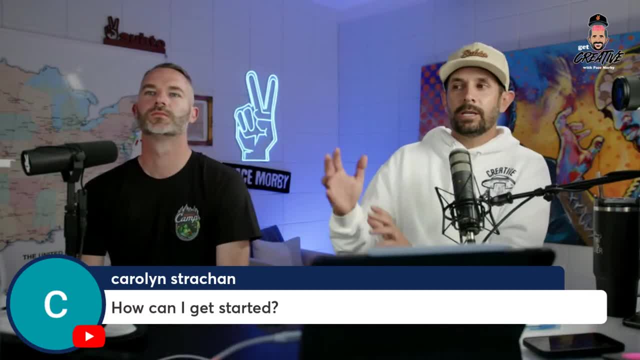 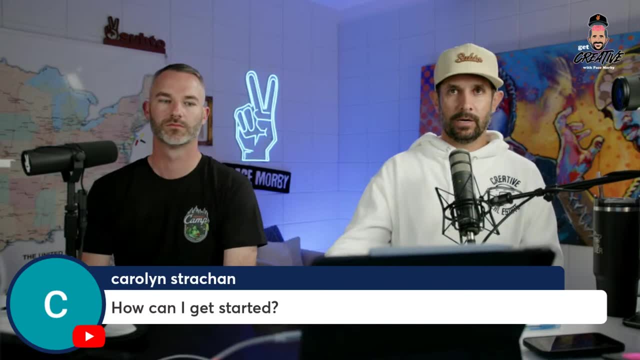 Okay, there you go. Boom boom, boom, boom boom. There's another video. So I, if I were you guys, I would not use. I would use section eight as one of my strategies And I would become a master of understanding all exit strategies. 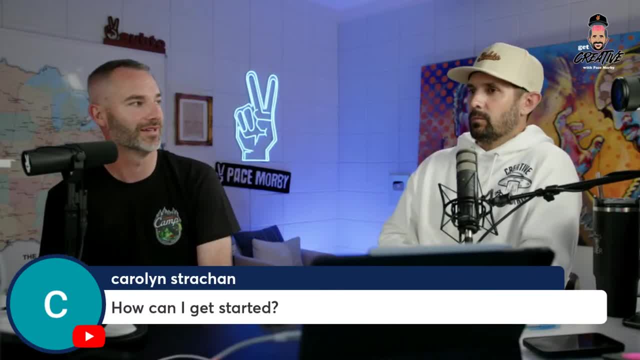 Here's what you're doing. when you guys do that, Your would you ever go play golf against me and only have a driver? Not if I was trying to beat you. Okay, Okay, Okay, do without, probably like a four iron. okay, the four iron is pat is uh section eight, just so you know. 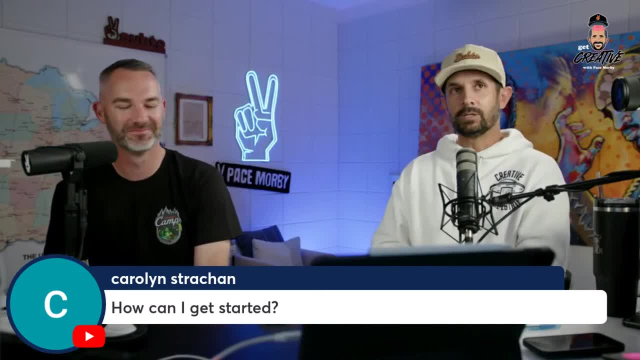 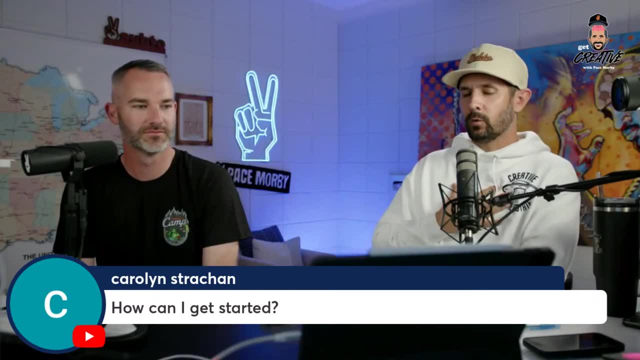 it's the one exit strategy i could do without and i could still beat you, take, take. it's not that i use my foreign a couple, you use your foreign, i think, a couple times. yesterday too, i hit my four iron like 210. the other day, had a great shot, actually overshot the hole. i was like dude this. 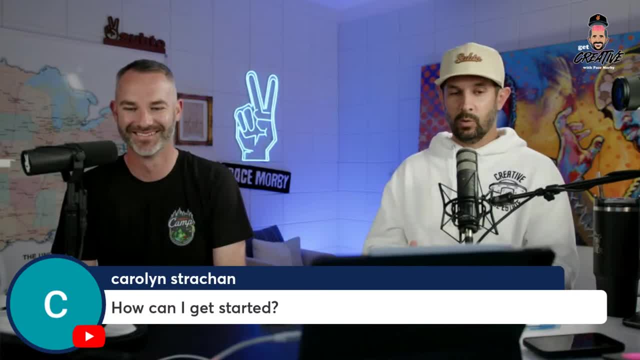 four: iron is pretty dope, but i'm telling you, it's the one club you would take out of your bag. it's the one club i would take out of my bag and still have confidence to beat somebody in a match. right useful. but there's better options. section eight: there you go. do i still want it in my bag? 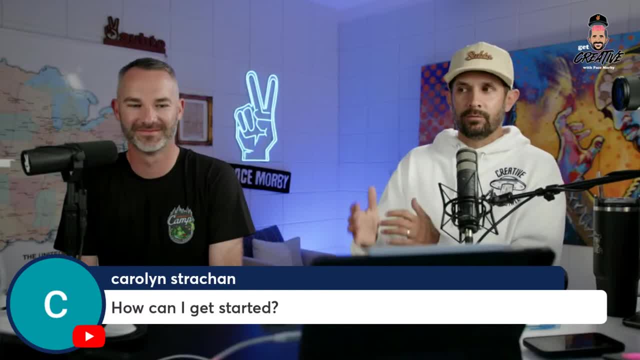 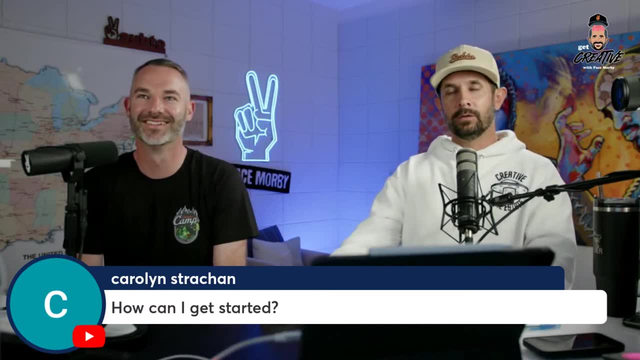 yes, but if you told me, take one exit strategy out of your bag, it's section eight. okay, the four iron of investing strategies. there you go, dang, that's a great analogy. um guys, thank you so much for coming in and hanging out with us tonight. it's a shorter episode than normal. i'm gonna go. 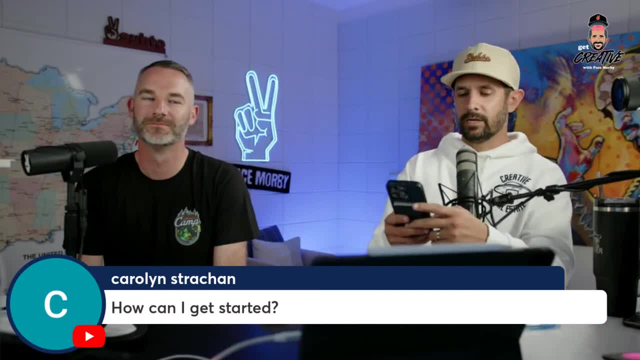 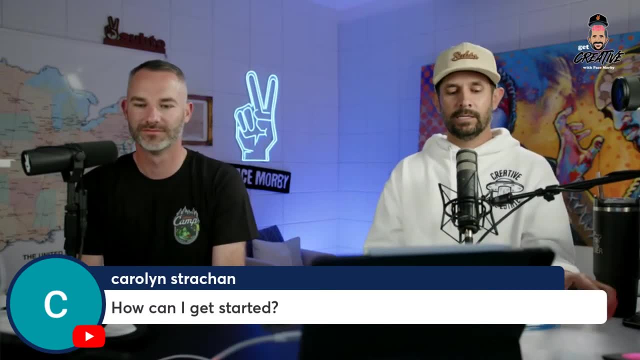 take uh jordan to dinner, if he'll. if he'll have me, we're gonna go get some tacos with some people and and um have a good time. by the way, if you guys are in arizona and you want to come and grab tacos, we're gonna go to taco boy in downtown tempe and we will be there. 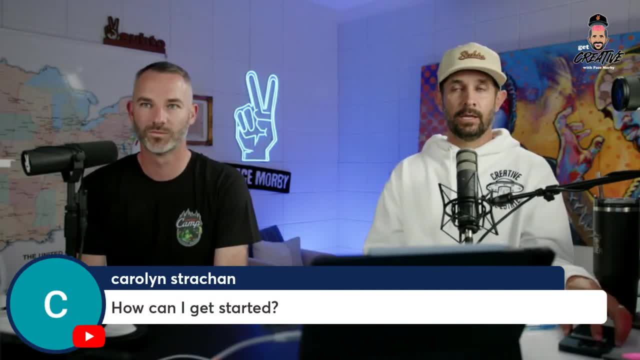 at 8: 30, so that's in about 45 minutes. i'm gonna go hang out with my girls for 15 minutes. he's gonna hang out with his girls for 15 minutes. we're gonna go down to taco boy and hang out. i look forward to seeing you guys tonight. thank you so freaking much um. by the way, we'll be back here. 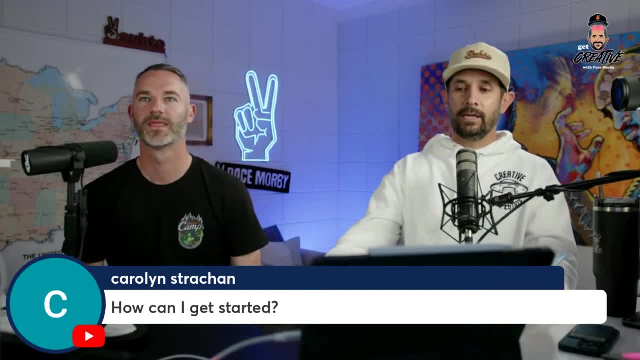 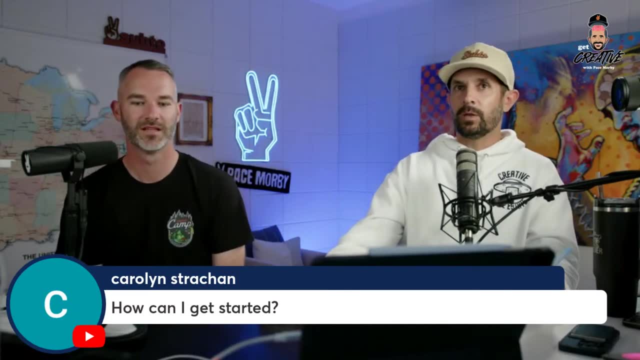 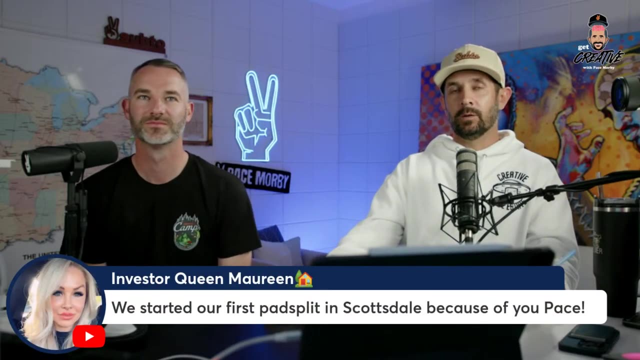 monday and anybody, i think, as of today, summit tickets are sold out. nice, i think. so i think we might have like three, four left, something very, very small. yeah, um, hey, there you go. investor queen marine says we started our first pad split in scottsdale because of you pace, thank you, thank you, i appreciate that. um, so if you guys do not have, 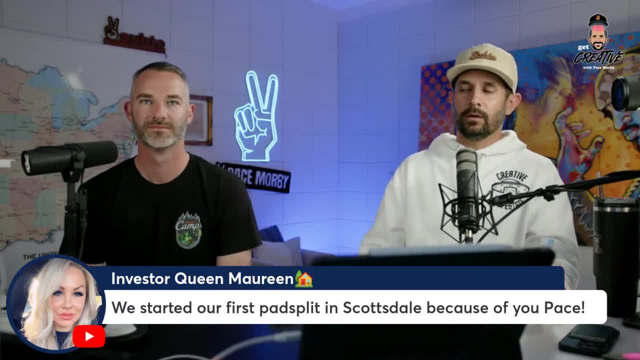 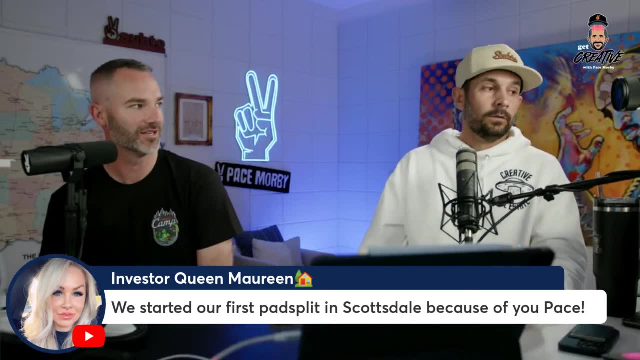 a ticket to squad up summit. it's next week, i believe we- uh, you sold three tickets today. i did. yeah, we got a little vip upgrade, so it's gonna be a good time. grant cardone, cody sanchez, vina jetty- the one that it will be the best speaker at the whole thing. there's two speakers. i'm really excited. 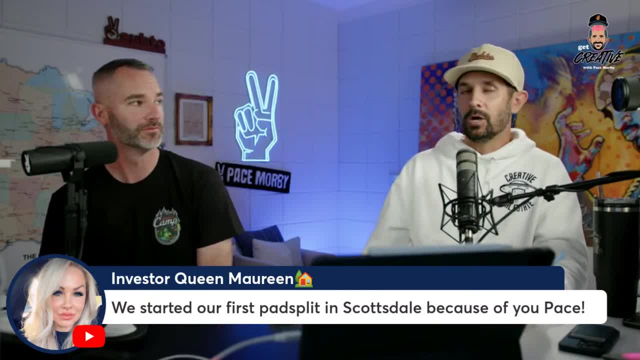 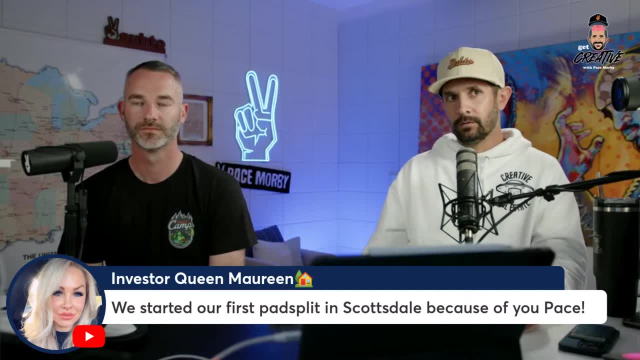 about jerry norton, jerry norton and donald miller. donald miller- yeah, i think donald miller will be one of the most important people you hear speak and he's on day one and he will help align you with your goals incredibly quickly. that's why we chose to have him on day one, so we can go through. 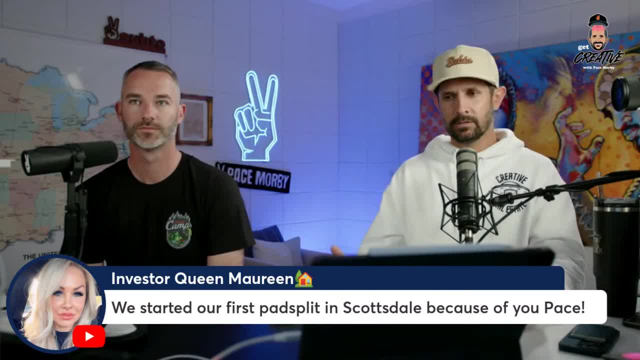 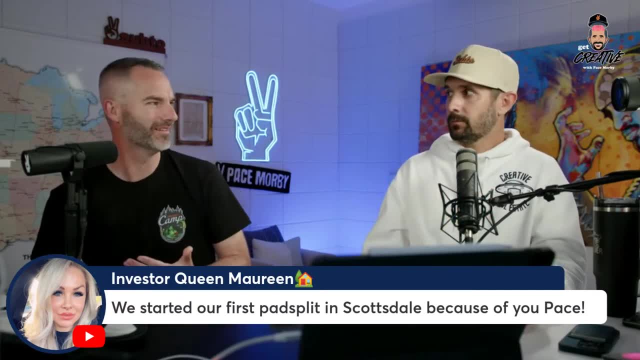 the three-day event with a cadence, and he will be a guy that he's section second speaker. i'm speaker number one, it's my event and i'm going to be the second speaker. i'm going to be the second speaker, i'm going to be the second speaker and the other guy is the main speaker, and then you're. 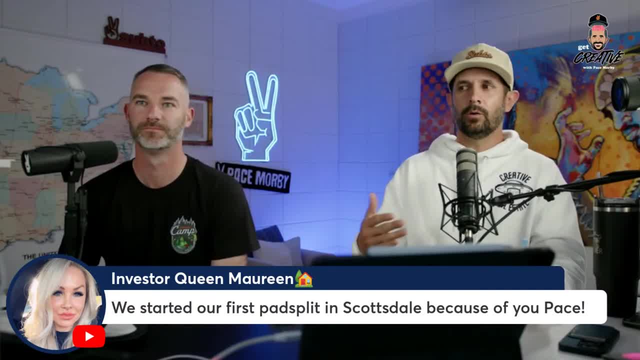 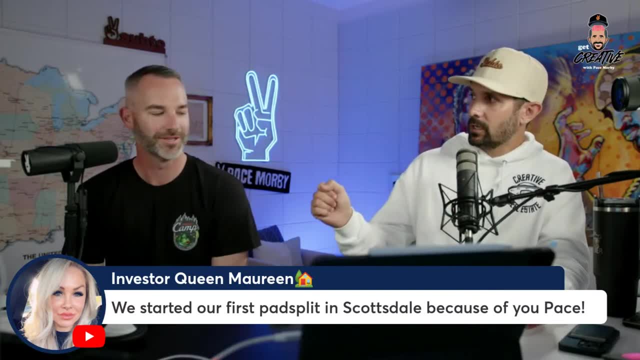 going to be the second speaker, and then you're going to be the second speaker and you're going to be the last speaker of the whole event. so, of course, and jamil jamil will speak two, maybe three times, i'll speak four times. cody sanchez once, uh, donald miller, twice actually he'll speak on stage. 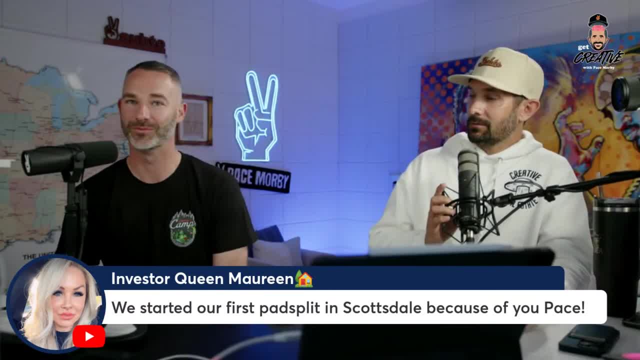 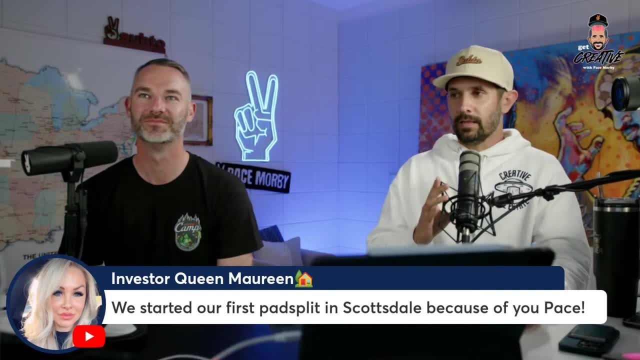 once and then in the vip room. that's a good job. you get to hang out with everybody in the vip. there's like dude, the vip room is going to be lit. it's gonna be good. i can't wait. it's like all your, it's a live event. i just don't. i don't believe in streaming live events. a lot of people can watch. 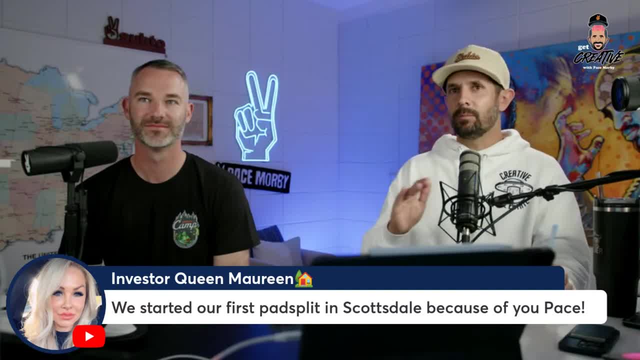 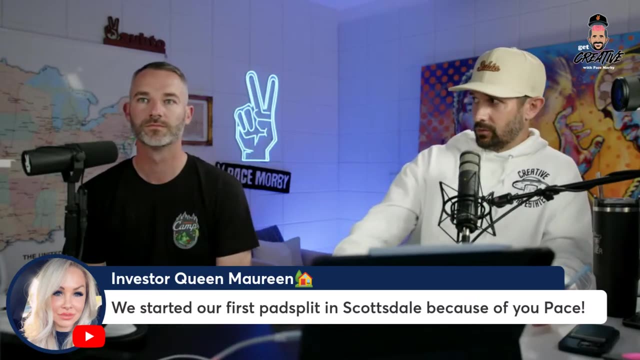 the replay, but the event. honestly, the best part of the event is the physical proximity to other people. so like streaming it to you guys is not really that beneficial. okay, so squadupsummitcom, if you guys don't have a ticket, i think it's sold out as of today. i think you probably sold the last.